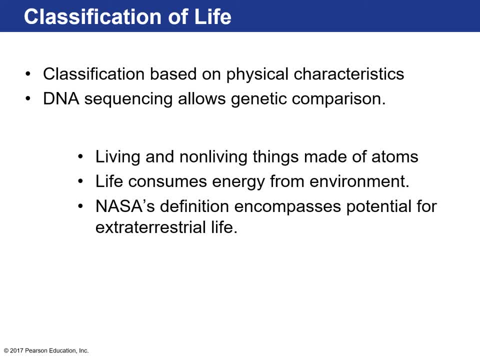 which closely resembles the classification based on physical characteristics, But there were differences between the classes, the physical characteristics, but they're all were some kind of adjustments to that. okay, it's hard to define life. life, things that are living, and things that are non-living are both made up of atoms. 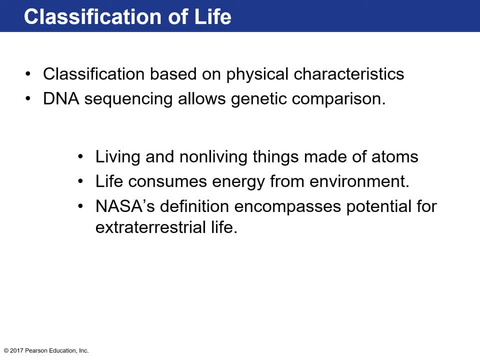 but how so? how do you distinguish something that's living from non-living? it's kind of harder than you think. one can come up with an idea that that perhaps living things consume energy from the environment. that might be a good working definition of life. but a car engine, for example, also consumes. 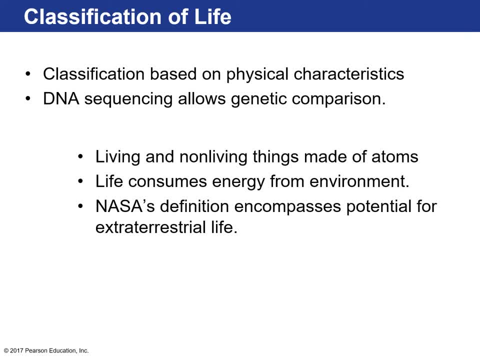 energy, so that doesn't really fulfill kind of like the distinction of living and non-living things. but car engines can't replicate themselves, they can't build themselves, so there's no reproduction in that. so that's, that wouldn't be a really good definition. NASA definition of life is that life is a self-sustained chemical system capable. 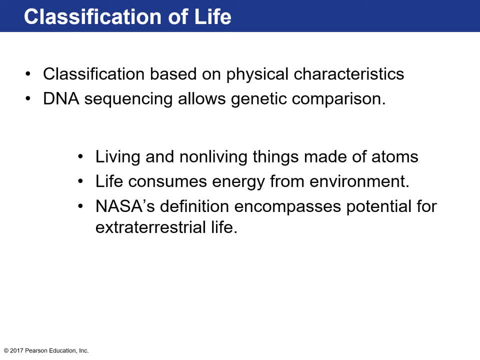 of undergoing Darwinian evolution. okay, and that allows for the existence of extraterrestrial life, although it's hard to kind of. if you're using that definition, you'd have to see multiple generations of organisms and witness some sort of genetic change and adaptation for it to be life. 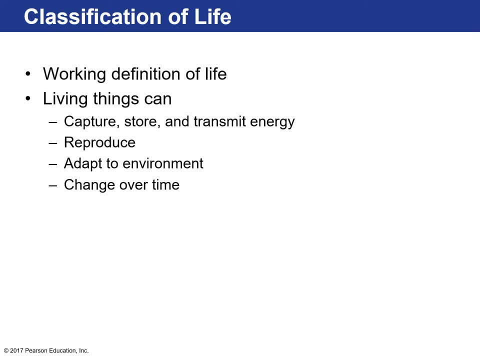 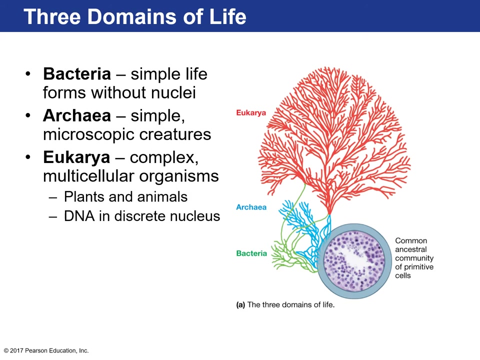 so really, the working definition of life really focuses on living things that can capture, store and convert energy and they're capable of reproduction, and that they can also adapt to our environment and change through time. all right, so there's three domains of life and all living things fall under these super. 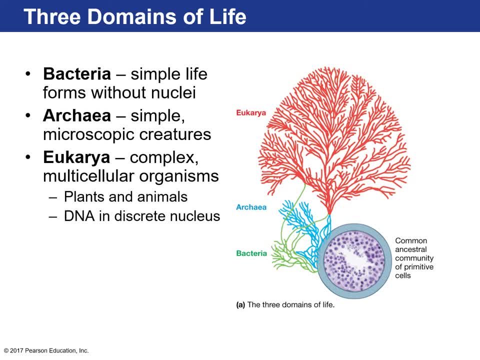 kingdoms. there's the domain bacteria, and that includes simple life forms with cells that usually lack a nucleus, and that includes bacteria, green non-sulfur bacteria and cyanobacteria, which is blue-green algae. then there's the domain archaea: those are really simple, microscopic bacteria, like creatures that 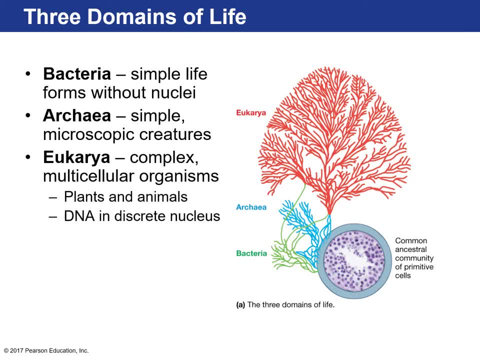 include methane producers and sulfur oxidizers. they normally live in deep deep-sea vents, so at rift valleys and mid-ocean ridges, deep-sea seeps. Then there's a domain, Eukarya, and Eukarya includes a lot of different complex organisms. 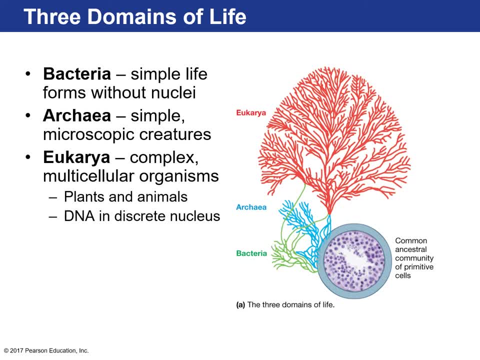 multicellular plants, animals, fungi, prosists, and it's a very diverse array of microscopic organisms that fit into that group, And the main component of Eukaryotes, or what distinguishes them from Archaea and Bacteria, are those domains of life. essentially is that Eukaryotes have DNA housed in a nucleus. 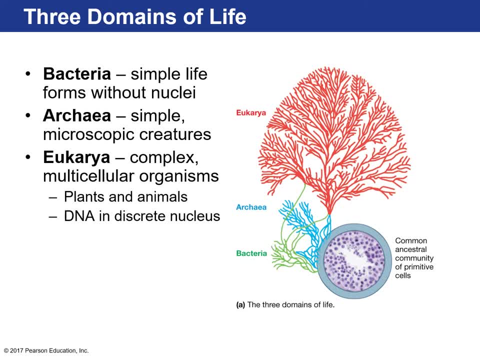 in their cells, and that's the main difference. So here are those three branches of life. This is Bacteria, all the different species that branch off from a common ancestor. This is Archaea, And then these are the Eukaryotes. 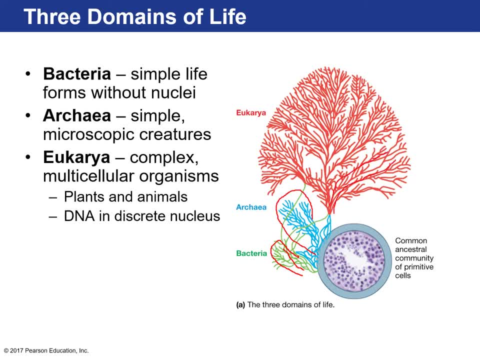 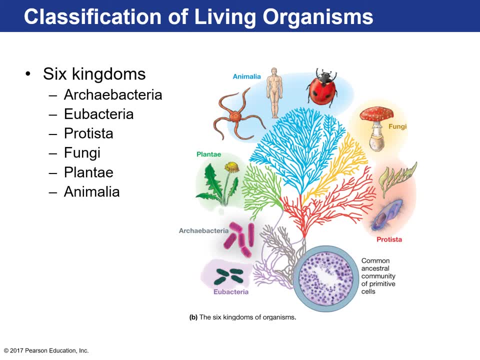 And these branches kind of move off into distinct organisms. So how do we classify the living organisms? Well, we classify them into six kingdoms, And those six kingdoms are pictured in this slide. Here are the Eubacteria, the Archaea Bacteria, kind of like the main superkingdoms. 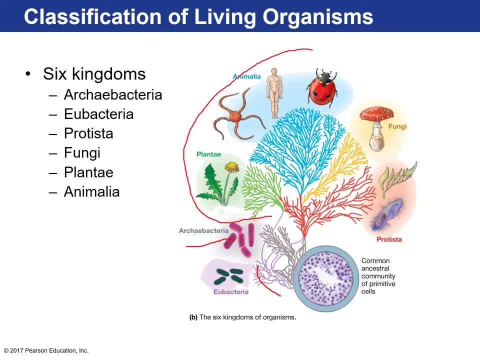 And then all of these are Eukaryotes, all in the same superkingdom. here We have Kingdom Plantae. This comprises of multicellular plants which photosynthesize, So that's kind of all the organisms that fall under this kind of subcategory. 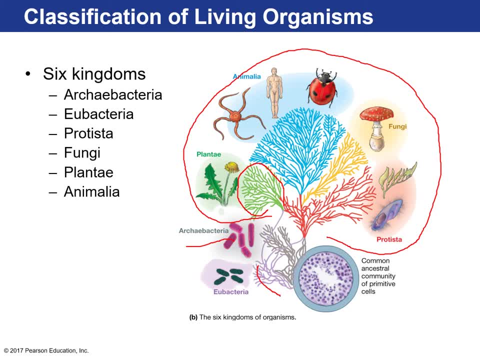 They can inhabit shallow coastal waters. They're also included in this- are photosynthetic marine algae And also land plants. Okay, They're vital parts of many coastal ecosystems, including mangrove swamps and salt marshes. Then there's Anamalia, which is this whole kind of kingdom here in blue. 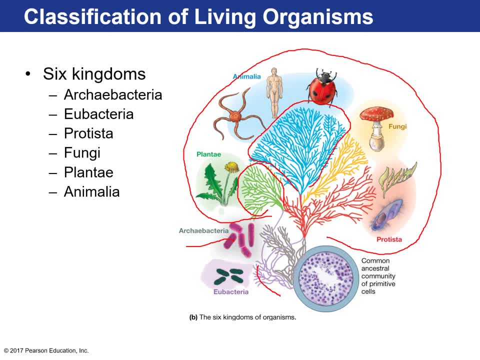 And that comprises of multicellular organisms. They range from simple sponges to really complex vertebrates, animals that have backbones, And humans are also part of that kingdom. Okay, Then there's fungi. Okay, That includes like over 100,000 species of molds, lichens. 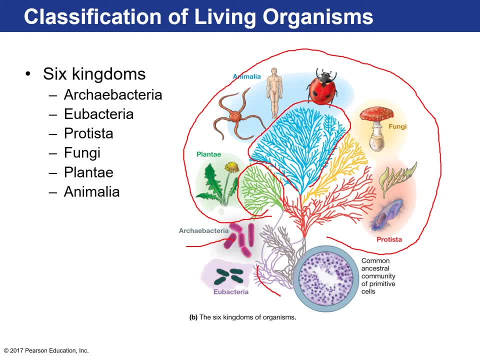 Fungi exist in all different types of environments. They also live symbiotically with cyanobacteria and green algae. Okay, So that consists, and again, also, we find them on land too. That's why you can see that picture of a mushroom. 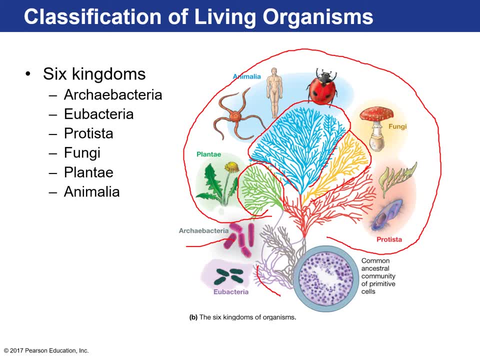 And then there are protists, and protists are diverse collection of single-celled and multicellular organisms that have a nucleus. It includes a lot of marine algae, photosynthetic organisms that can either be microscopic or single-celled. We refer to them as protozoans. 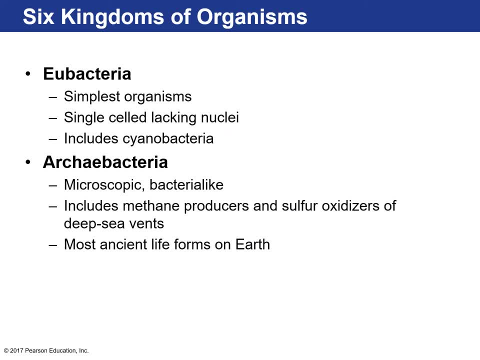 Okay, So here's Eubacteria. Those are the. this is the kind of skip glossed over them, but they're very simple organisms. They're single-celled and they lack nuclei. That's how they're different from Eukaryotes. 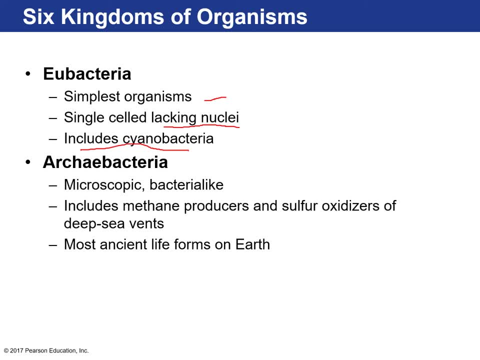 And that includes cyanobacteria, So Archaea bacteria. they're microscopic, They're a lot like bacteria, They just differ slightly, And it's actually believed that they might be the first organisms to exist on earth, because they exist in kind of deep sea vents. 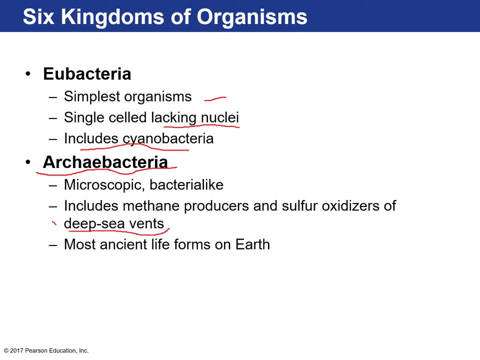 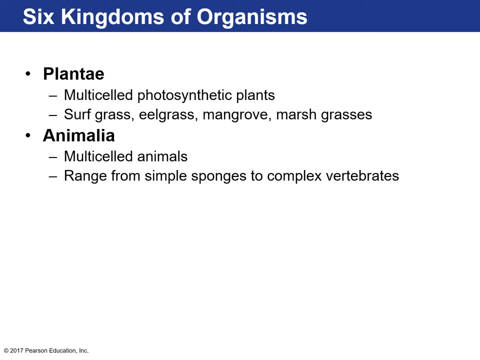 And this is an environment that was probably prevalent in early earth. Okay, And they can live. They can live, you know, kilometers below the crust, under harsh conditions. Okay, So I've talked about the plant group. All right, Surf grass, eel grass, mangroves, marsh crashes- include that? as it relates to oceanography, 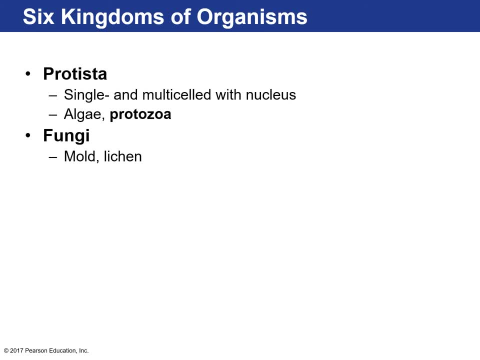 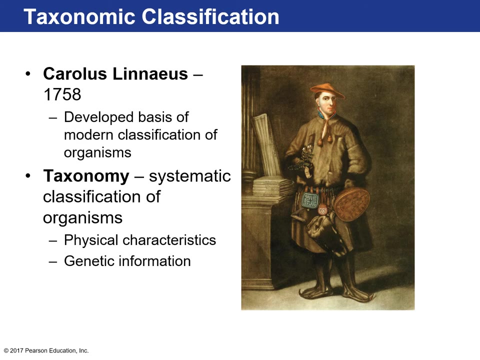 Okay, Fungi- I mentioned that they're mold and lichen. protistas are single and multi-celled nucleus algae. Okay, All right. So how did this initial classification go? Okay, So how did this classification kind of show up in the scientific world? 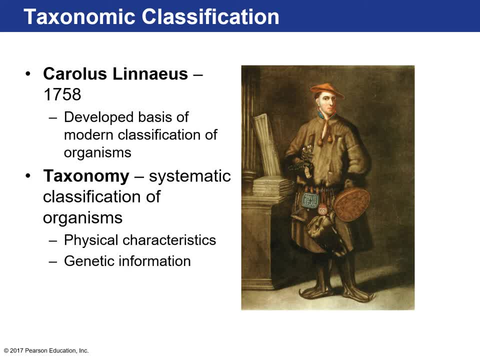 Well, we'd have to thank the Swedish scientist Carlos Linnaeus in 1758.. He's the one who kind of came up. He was a Swedish botanist, right, He's the father of taxonomic classification. Okay. 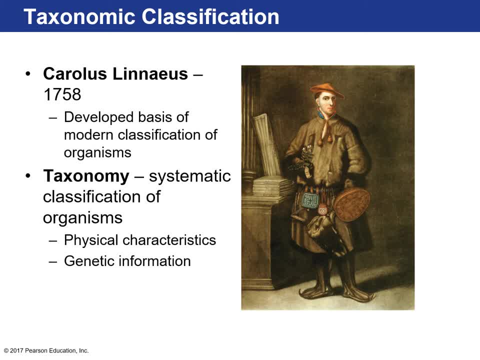 So he developed the modern form of classification. Guys, look at his scientific Batman belt. Look at all those gizmos he had on him. Probably had a lot of them. Probably had a bunch of butterflies in there. Okay, I don't know. 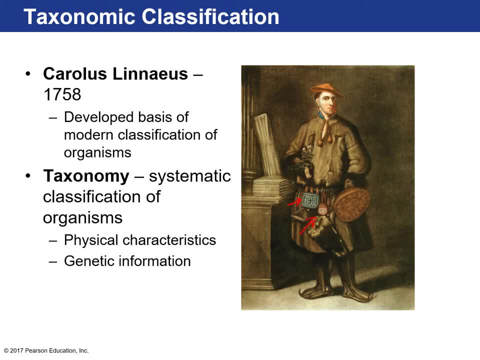 Caterpillars, all different types of scientific instruments, can do anything out there in the field. He probably had dowries thrown at him from all different sides. Linnaeus, Okay, And so he based his taxonomy on physical characteristics of organisms. 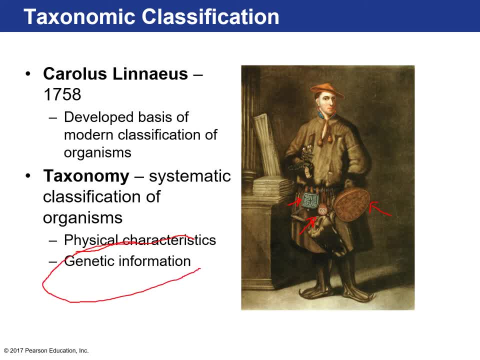 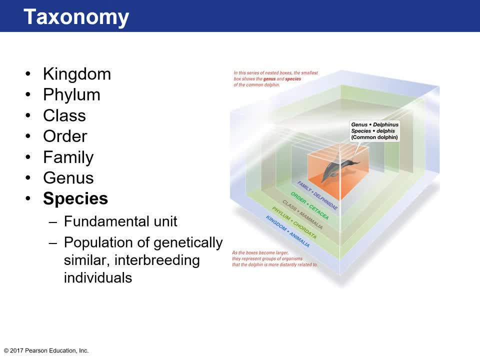 Okay, Later on it was adjusted with the newly acquired genetic information, Okay, Okay. So what the taxonomy essentially is is it kind of determines the relationships amongst all living organisms, And he created this system kind of like to like narrowing down specific species of organism. 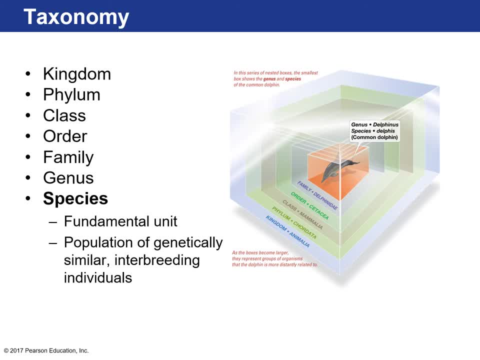 Okay, So you start off with a less specific grouping, which is the kingdom- And we talked about those six kingdoms- And then you move down to the phylum, Then the class, Then the order, Then the family, Then the genus. 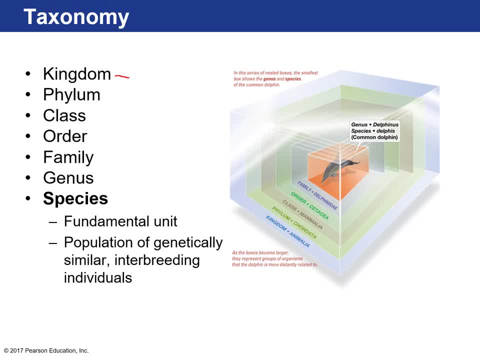 And then the most specific grouping would be the species name. Okay, And that's that fundamental unit. Okay, So a species is defined as a population of genetically similar interbreeding individuals. Okay, So, for humans, we're homo sapiens, sapiens. 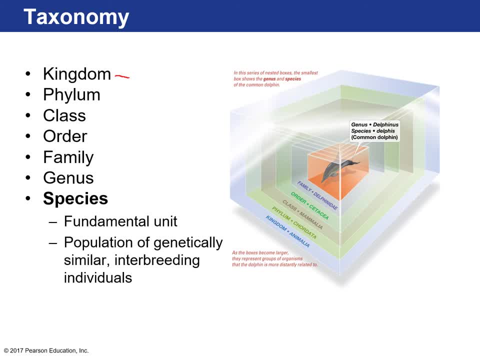 We can all if we're all human. there are no other subspecies or different species of humans on earth today. There were in the past, But, yeah, we could all potentially reproduce and have children because we're all in the same species. 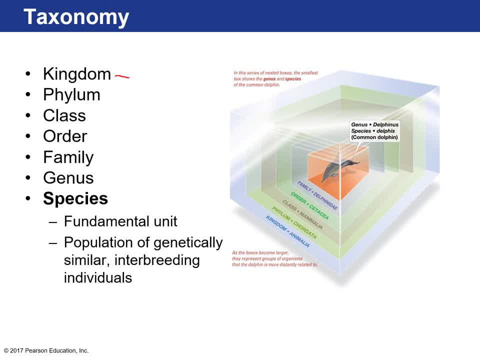 Okay, So for a dolphin, which it's a common name is dolphin- Okay, But it's species is Adelphys- Okay, And it's genus is Delphinus- Okay, And it's part of the kingdom of animalia, which includes us. 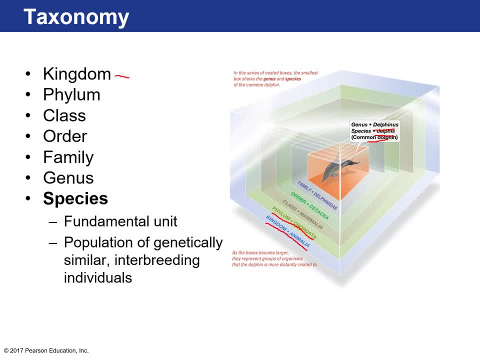 It's phylum is Cordata, Meaning it has a backbone. Okay, That also includes humans, So we're in the same phylum. It's class is Mammalia, So that's where it differs from amphibians and reptiles. 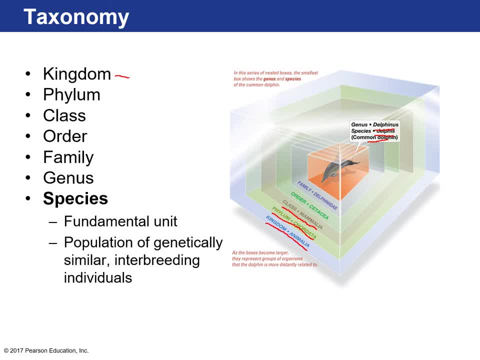 Okay, But again, humans are also mammals, So we're also in that same group. but once it gets to the order, that's where it differentiates from humans. It's a cetacean. Okay, Those are essentially marine mammals. 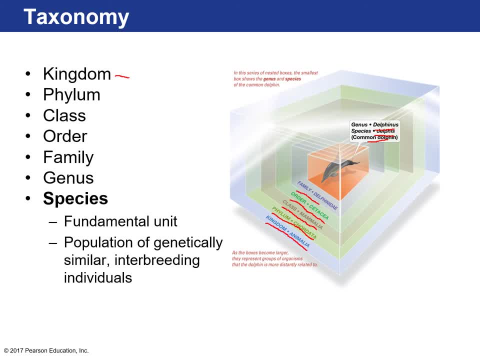 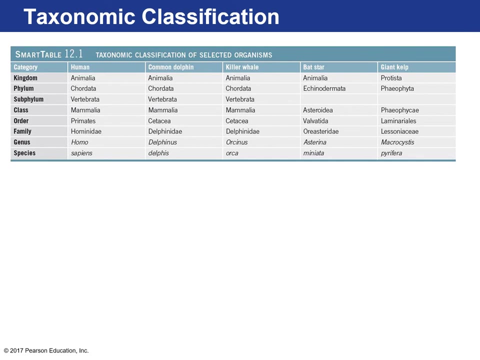 So that includes whales, And then, more specifically, It's family is Delphinidae. Okay, And so those are all the different species of dolphin. Okay, So that's how the taxonomy of ocean organisms goes around. Here's some more examples of it. 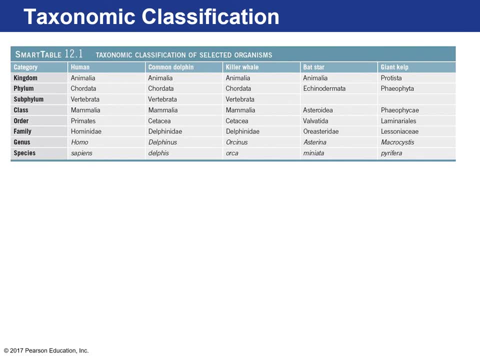 Here's Homo sapiens, Right, So we're phylum Cordata, sub phylum vertebrata, Our class is Mammalia, We're primates, Okay, So that's where we differentiate from dolphins, And then our specific family is Homo sapiens. 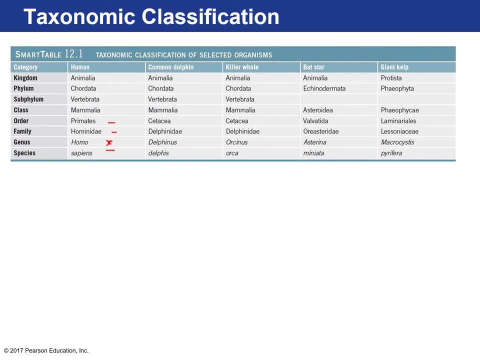 So when you refer to an organism, you give it by its genus and then its species. Okay, Here's the killer whale, Very similar to the dolphin. The only difference is its genus and its species name, So they're in the same family. 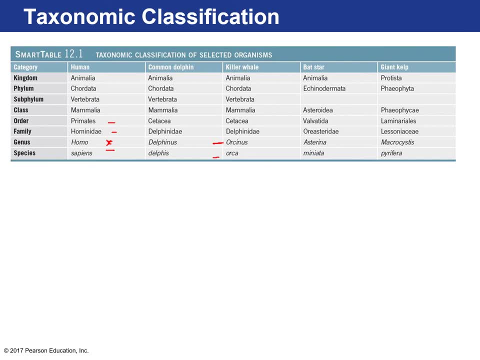 Okay, And then we can look at like a protist, for example. that would be completely different. Down to its kingdom is different. Okay, All of these family order and class are all different, Okay, So how do we? 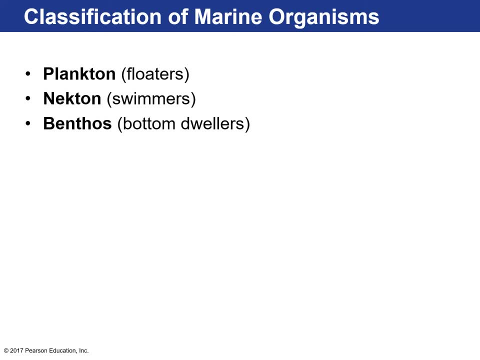 The classification of marine organisms is based on kind of like: if they can swim, if they can float or if they're just hanging out at the bottom of the ocean floor. Plankton refers to organisms that can actively choose where they want to swim to. 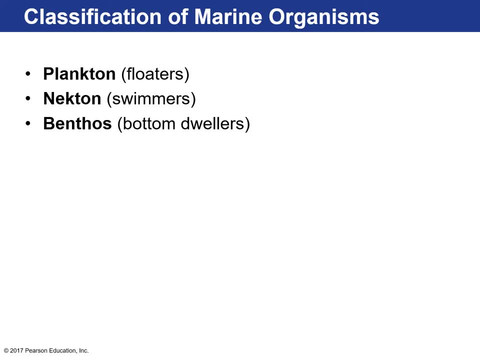 They just float around, And so their goal is, Typically, they want to stay in the upper 100 meters of the ocean surface, because that's, on average, how far sunlight can penetrate into the ocean water. So they want to float around in those layers. 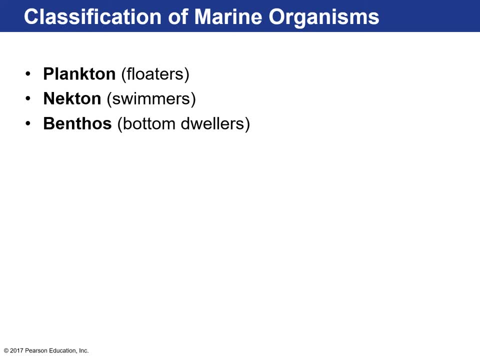 One, because either they're autotrophs or they photosynthesize to produce their own food. In that case, they want to be in the sunlit layers, Or, if they don't do that and depend on eating other organisms, they want to eat the organisms. 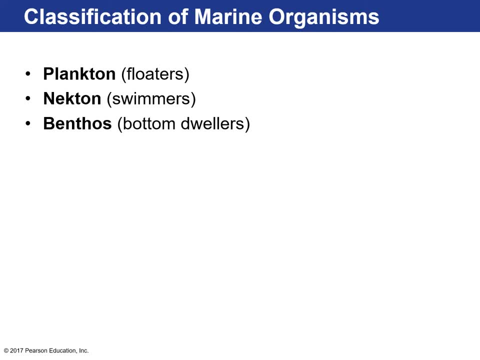 that photosynthesize, So they want to be in that area of the ocean. Okay, Plankton are active swimmers. They get to choose where they want to go. They can swim to different coastal waters, different depths, surface shallow areas. 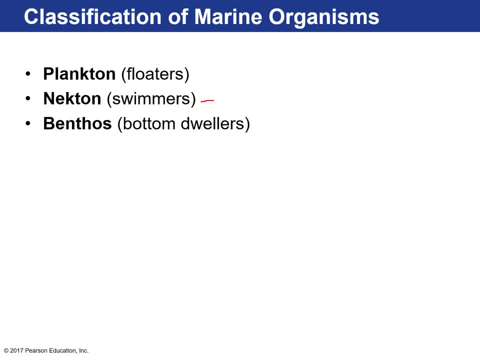 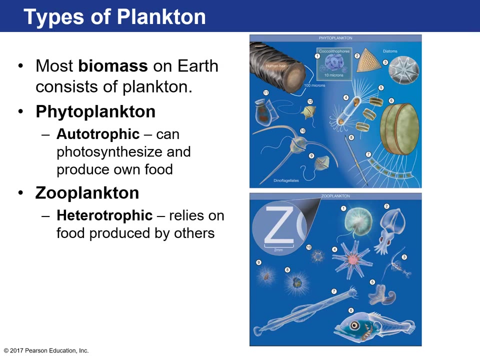 And then benthic organisms or benthos or bottom dwellers, organisms that are either attached to a substrate in coastal waters or even deep waters, or they kind of crawl along the bottom of the ocean floor. Okay, So that's the first one. 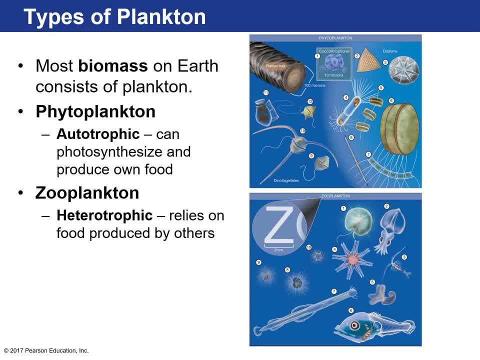 Okay, So let's talk about the different types of plankton. Plankton make up the majority of the biomass on Earth. Okay, If we're talking about the oceans, right, they cover 71% of the Earth's surface. Plankton are kind of like the grass of the ocean, so to speak, because they're algae. 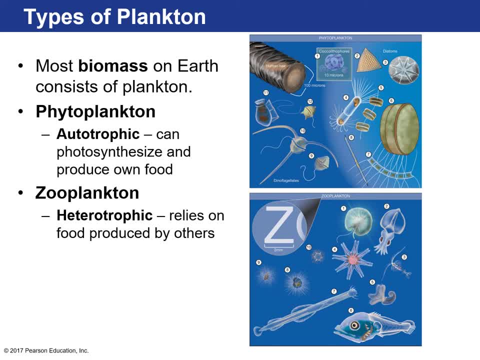 that kind of float on the surface or the sunlit layers of the ocean, And so if you were able to put all those organisms on a scale, they would outweigh all other organisms on Earth. Okay, Phytoplankton is what I was referring to as the grass, because they're autotrophic meaning. 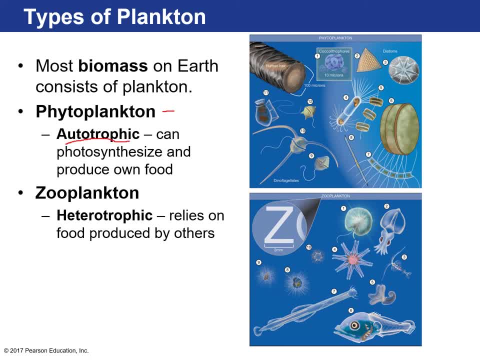 that they can produce their own food. They can photosynthesize, So they kind of just float around and create their own food. Here are some examples of some. Okay, This is the width of a human hair, So you can kind of understand scale here. 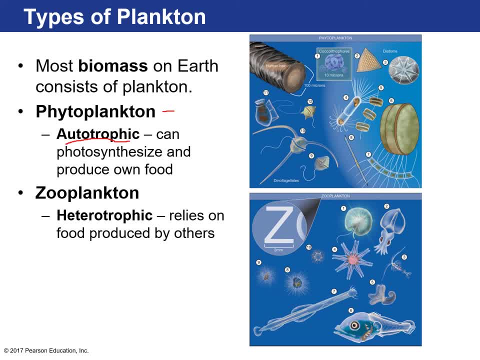 These are coccoliths. These are pretty small. Okay, These are organisms that create these plates around. They're single-celled. These plates are made of calcium carbonate and they photosynthesize. And then there are diatoms right here. 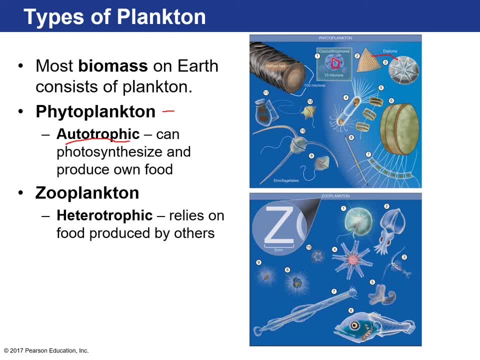 These two are diatoms. They also photosynthesize and they create their shells out of silica, which can accumulate as biogenesis at the bottom of the ocean. Okay, Great, Okay. Then these organisms over here, 9 through 12, okay. so these organisms, these are dinoflagellates. 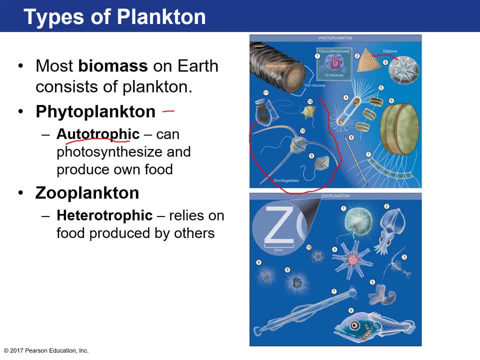 Okay, These are also phytoplankton. Some dinoflagellates are responsible for the red tide, Okay. And then, if we go down over here, these are zooplankton. Okay, So zooplankton are slightly larger than phytoplankton. 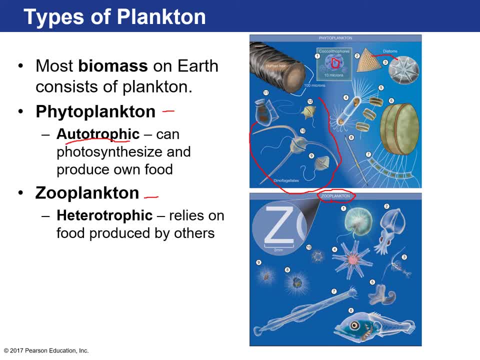 And zooplankton can't create their own food. They rely on food producers or running into them, bumping into them in the ocean and then just gobbling them up, essentially, And so they rely on eating these guys, essentially. 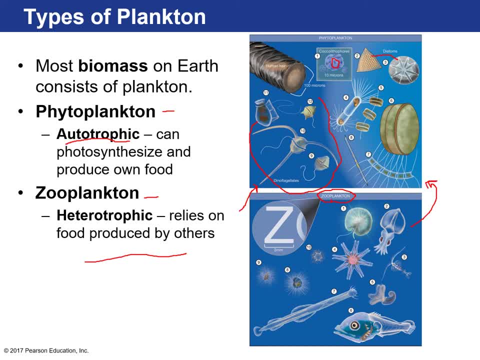 So these are the kind of first level of organisms that eat, the kind of The autotrophs or the The autotrophs, The autotrophs, or the bottom of the food chain. let's put it that way. 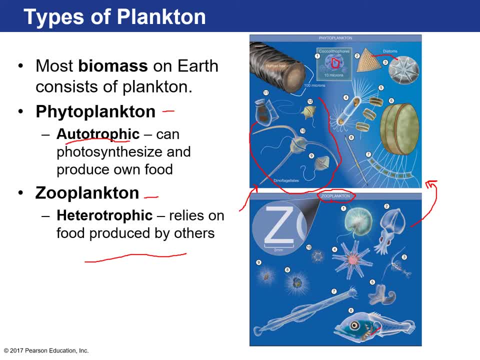 Okay, And that includes squid larvae, fish larvae, arrow worms, foraminifera, okay, foraminifera are these organisms here? Here's the arrow worm. fish larvae, krill. okay, here's the squid larvae, Okay. 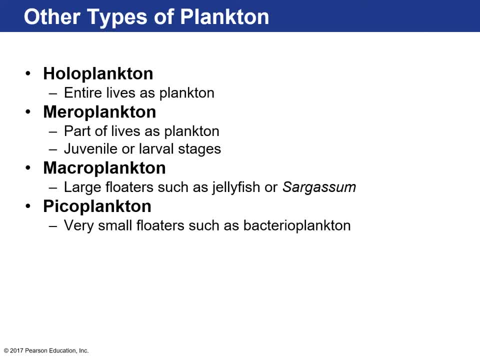 So those are all types of zooplankton. All right, there are other types of plankton organisms that just float around. Holoplankton refer to plankton that are essentially plankton. their whole lives Like they don't. 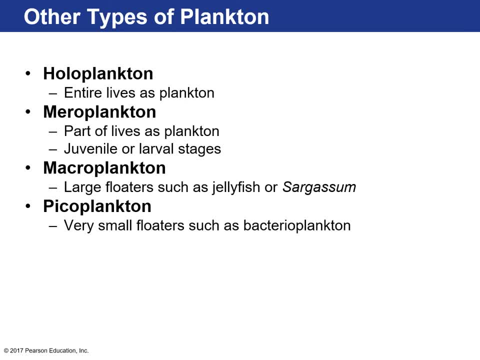 They can't ever actively swim. Miroplankton refer to organisms that live part of their lives as plankton, mostly in the larval or juvenile stages, but when they get larger then they become nektonic and they can actively swim. 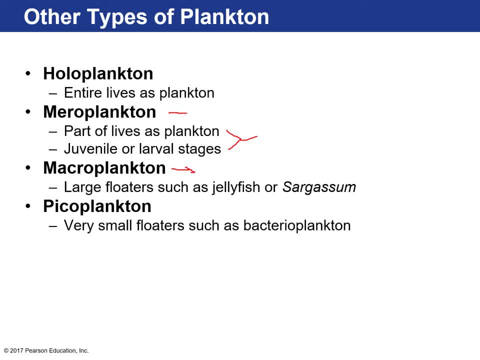 Macroplankton. These are larger organisms that float around or don't actually swim. Okay Okay, They don't actively swim. That includes jellyfish, or sargassum. That's an algae in the Atlantic that often washes up on our East Coast beaches. 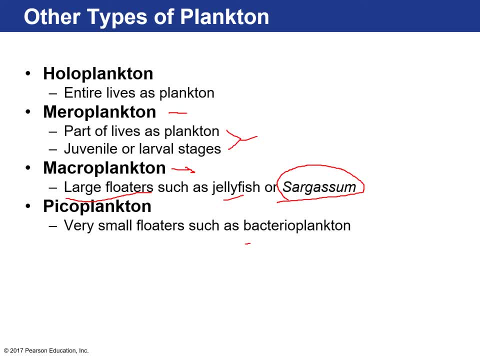 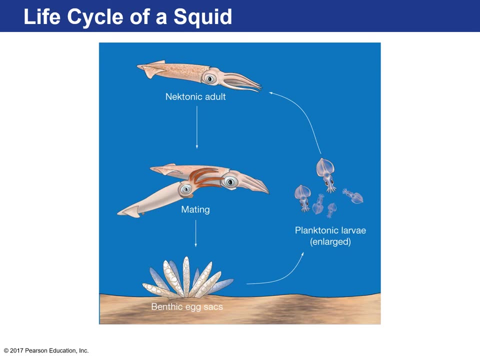 Okay, And then there's also plankton that are really really small bacterial plankton, Very small floaters. It's only until recently that we've actually found them in ocean water because they're so small. Okay, So here's an example of an organism that lives in all three kind of different. 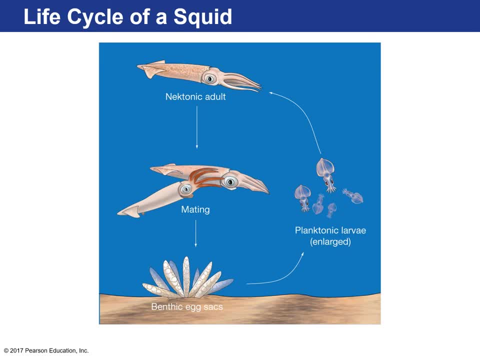 Phases A squid Initially. when they're egg sacs they're benthic because they're attached to the ocean floor. When they hatch they become larvae, and larvae can't really actively swim, They're just carried around by the currents. 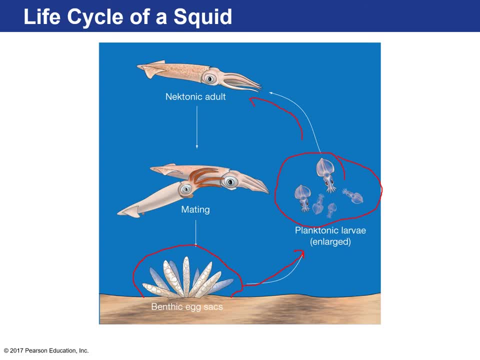 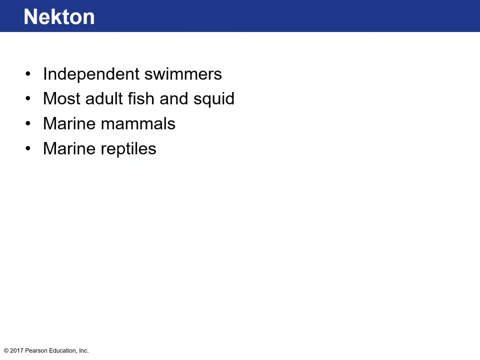 So that means they're planktonic, but once they grow big enough, then they're nektonic. Okay, And they can actively swim wherever they want to. Okay, So nekton are independent swimmers. Okay, These guys. this is most adult fish and squid, marine mammals, marine reptiles. 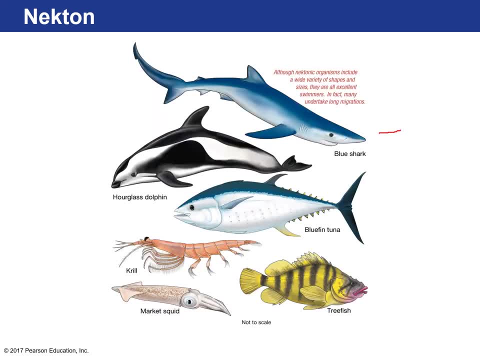 Let me show you some examples of those. Okay, Here's a blue shark, hourglass dolphin, a bluefin tuna, huge hunter in the ocean. We have krill squid, a tree fish, any fish that you would see in coral reefs. 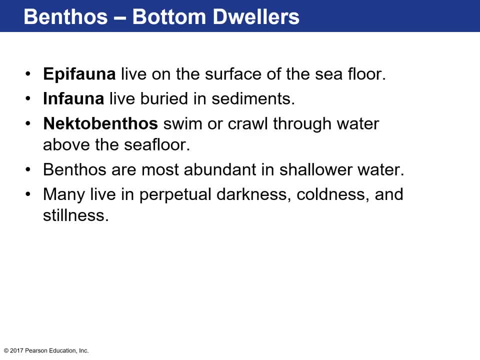 Those are all nektonic organisms. Okay, Then the bottom dwellers. there's a few different types. Epifauna are benthic organisms that live on the surface of the sea floor. Infauna are ocean organisms that are buried in sediment. 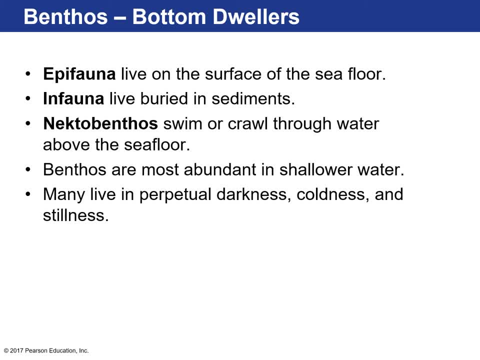 I'm sure perhaps you've done this, where you've gone to the beach and you've dug out handfuls of sand and you might see sand fleas or little crabs or sand dollars. Those are examples of infauna- Okay, Nectobenthic organisms. 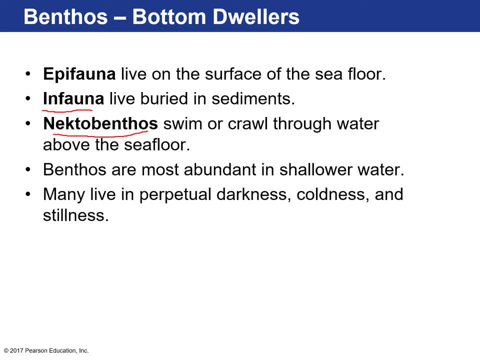 Okay, They swim or crawl through water above the sea floor. Okay, And benthic organisms are most abundant in shallow water. Okay, And this makes sense because their food source typically are organisms that rely on the sun to produce food, So that very first portion of the food chain and in shallow waters, the entire water column. 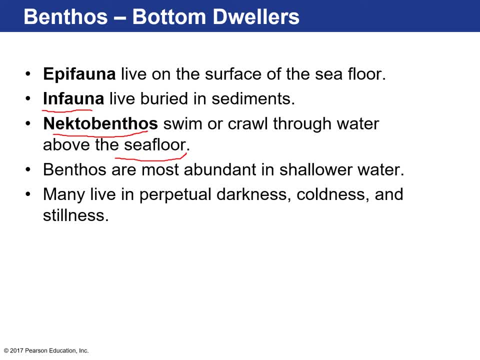 is lit up by these, By sunlight, Okay, But many benthic organisms do live in perpetual darkness, and that's in essentially any area beyond the continental margins. Once you go beyond about 400 meters, then it's perpetual darkness, Okay. 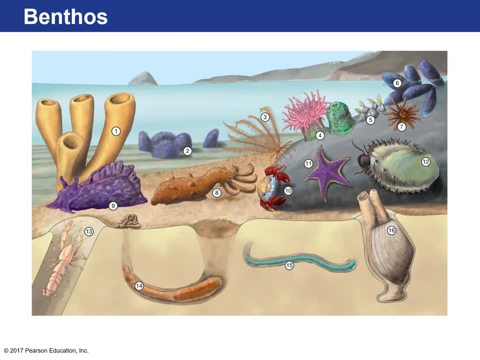 So here are some examples of benthic organisms: Okay, We've got sponges as number one. Okay, Or coral, Okay, Sea slugs, Okay, Mussels, Sea stars. Okay, Anemones, Okay, Crabs. 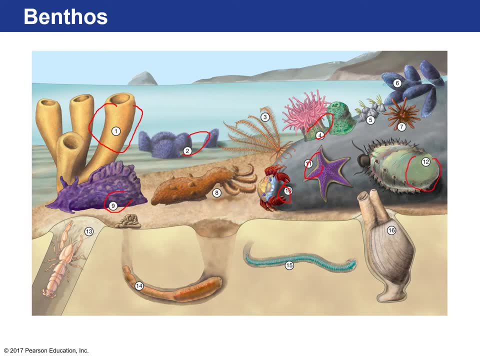 Okay, This is an abalone over here. Okay, I have a sea urchin. Okay, I'm sorry, Here are mussels. Okay, Number five are barnacles. Okay, So that's over here. Okay, Number 16 is an annelid worm. 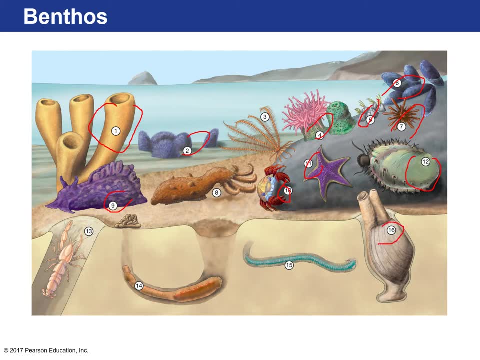 Okay, Sometimes you can see these at fish markets. Okay, Number 14 is a lugworm. Okay, So that's over here. Okay, Number 16 is an annelid worm, So that's an infauna. Okay. 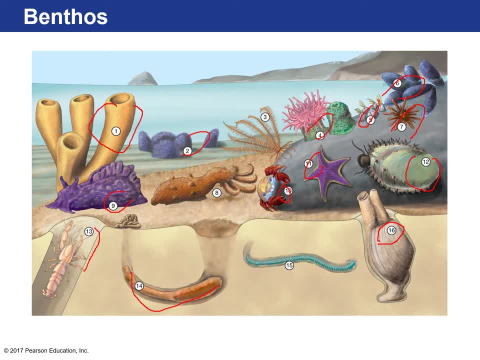 13 is a ghost crab. Okay, Because it hides up in the sediment. That's another infauna. 15. I'm sorry, 15 is the annelid worm. This is the clam. 16 is the clam. 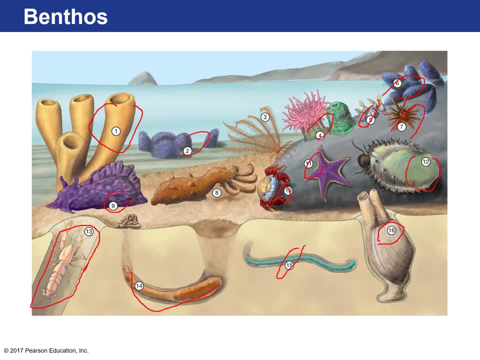 That's what you see at fish markets. Okay. Number three is a crinoid over here, And this is an anemone. Okay, So let's talk about hydrothermal vent communities. These are anemones. Okay, And this is an anemone. 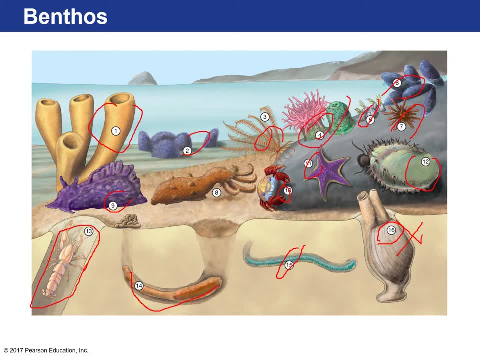 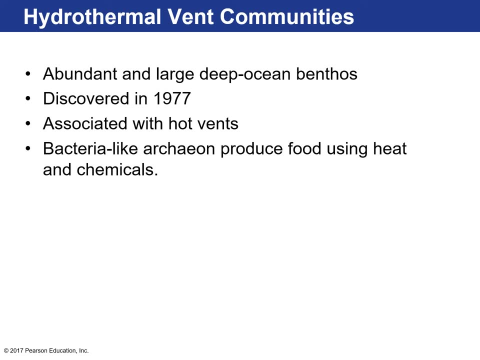 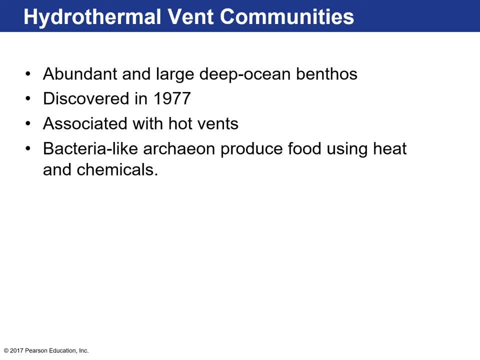 Okay, They were discovered in 1977, once we had submersibles with cameras go down to areas near mid-ocean bridges And so when they went and explored those areas they actually found really hot vents that would spew out really hot water. 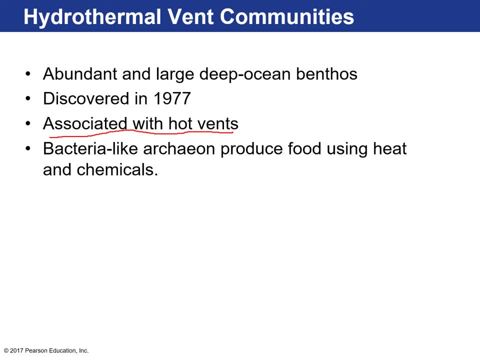 And they found life. That is kind of Okay. huge misconception that oceanographers had for the longest time is: they thought that ocean life, the basis of ocean life, is autotrophic organisms living in the upper layers of the ocean. so they figured that in perpetual darkness at 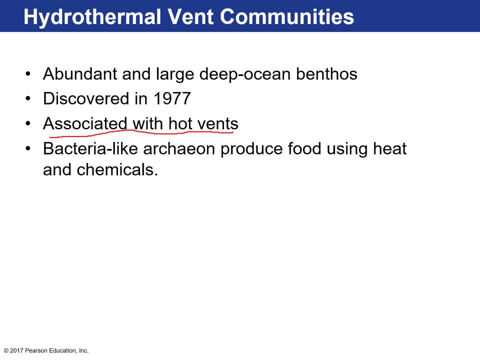 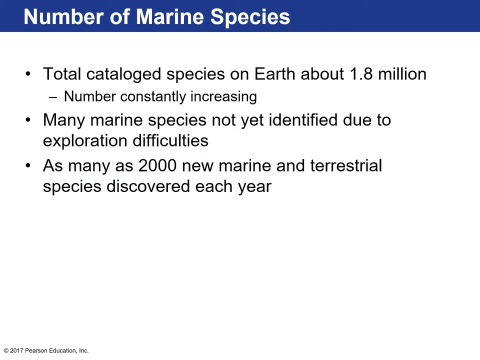 the bottom of the sea floor, where sunlight doesn't reach that, there would be no life. but they were wrong and they didn't realize that the basis of the food chain there is this bacteria, like our key in organism that produces food using heat and chemicals that are coming off of these hydrothermal vents. okay, I. 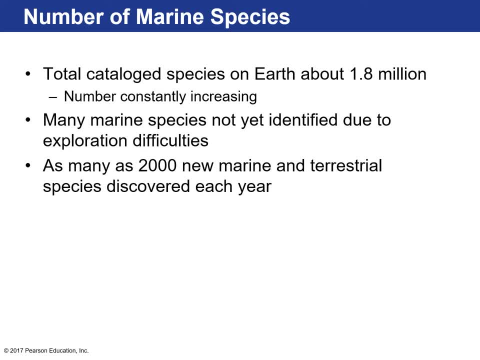 think we'll get into it a little bit in more detail. a little bit, but essentially they live within the tissues of a lot of the sponges that are surrounding the vents, and then they provide sugar for those- you, I- organisms and and essentially they found crabs and clams at those depths. 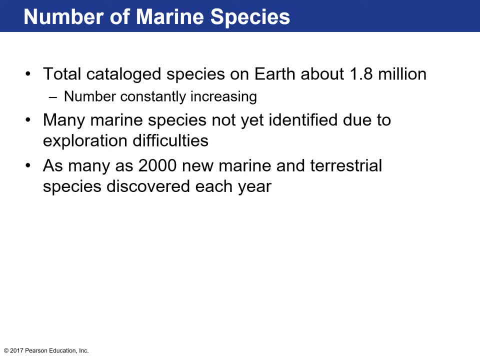 which are, which was pretty amazing. so life can, life finds a way. okay, all right. so let's talk about the number of different marine species that exists. the total catalog species on earth is about 1.8 million, which constantly increases because we start to discover new species. many marine species haven't been 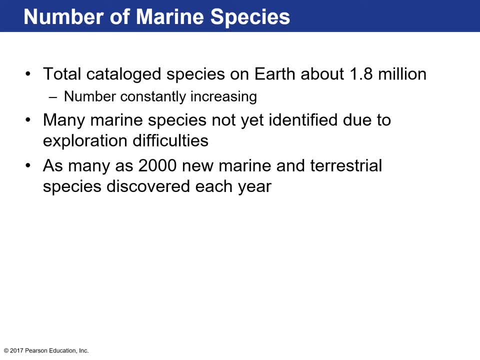 identified. because of exploration difficulties, it's tough to get to the bottom of the ocean. okay, and there's as many as 2,000 new marine and terrestrial species discovered every year, so you could be one of those people discovering new species. now there are more land. 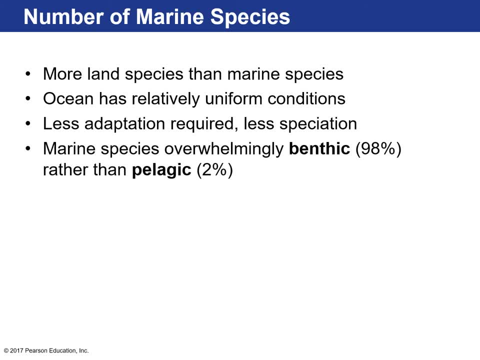 species on earth and there are marine species, and the reason is because land has more variety, okay, and organisms can adapt to that variety. they can find their little niche in that variety. the oceans are largely very similar. the kind of different environments of the oceans that vary are usually coastal waters. 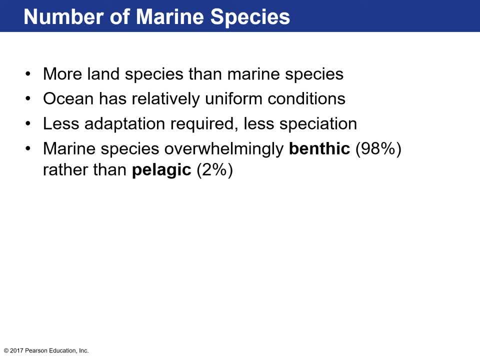 because of influx of fresh water, so varying salinity, varying temperature and also varying depth. so you see different, a lot of different environments close to land, but the open ocean is in the middle of the Indian Ocean. those conditions are very similar to the open ocean in the Pacific and the Atlantic, so those 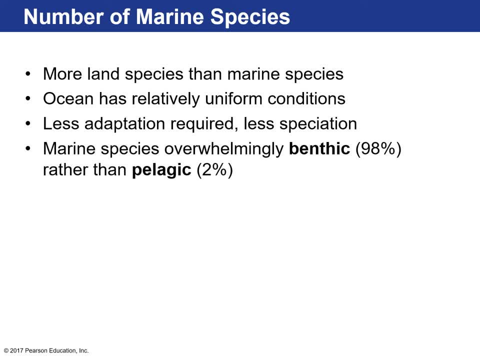 environments are very similar. they don't change that much. so the marine organism, organisms that encompass those environments, can be there or anywhere, there's not much difference. but if you go on land, you've got mountains, okay. you've got deserts, you've got swamps, you've got forests, you've got temperate. 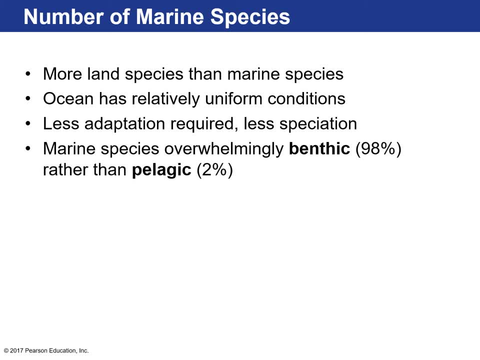 forests, you have the Arctic. there's a big variation in landscapes, temperatures, humidity, rain elevation. all those things contribute to organisms adapting to those specific environments, which leads to different types of species. so in the ocean, less adaptation is required and that leads to less speciation. okay, and 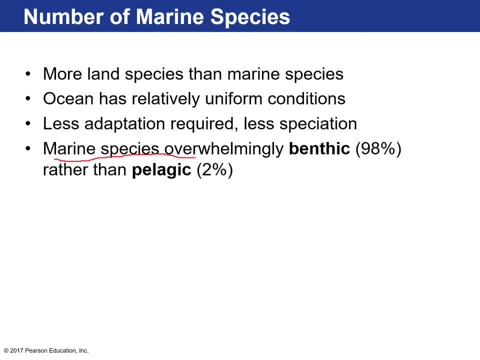 to that fact, marine species are overwhelmingly benthic. this is the number of different species, not the number of different organisms. so if you were to consider the different species- benthic meaning bottom dwellers or pelagic meaning the open ocean- they're far more different species of benthic organisms and there 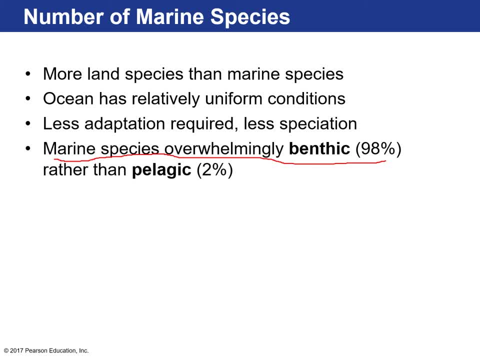 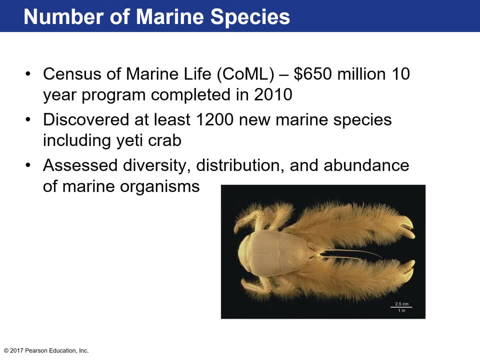 are organisms that roam the open ocean. okay, it's a 98 to 2% comparison. okay, there was the census of marine life. okay, it was a project: 650 million dollars were put into a program that was finished in 2010, and the purpose of this. 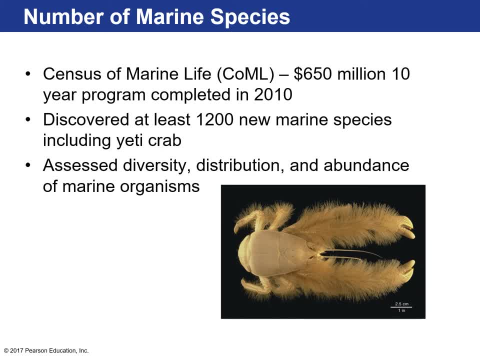 project was to go out and find new marine species, specifically a lot of times looking in the deep ocean floor, and they discovered a lot: 1,200 new marine species- okay, including the Yeti crab which is pictured here. it's called the Yeti crab because look at those hairy arms over. 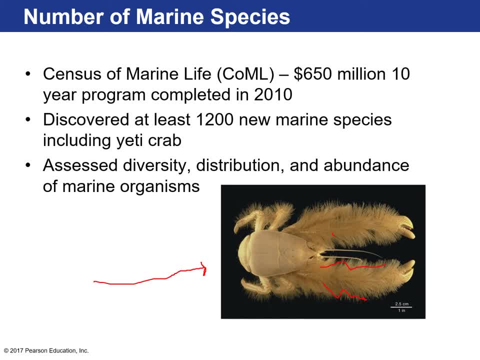 there. sorry, that was my Yeti impersonation. I don't know what a Yeti sounds like anyways. so what this project did is assess the diversity and the distribution of marine organisms. so highly successful, they found 1,200 new marine species, which is pretty crazy, okay. so here's the 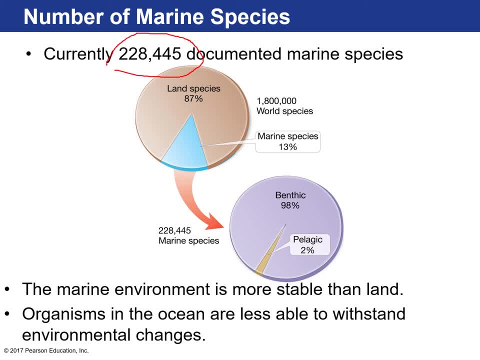 currently documented 228 445 species. okay, marine species specifically, so that only makes up 13% of the world. okay, most of it is different land species. so the marine environment is more stable than the land environment and that's why speciation isn't necessarily a requirement for the organisms in the 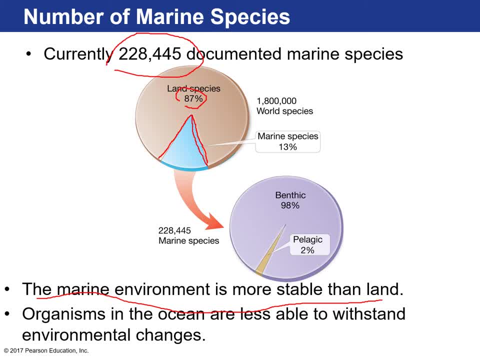 ocean, because that's all very specific and we just found- they found- that the population of marine species is 1.2 million, called. it's pretty crazy. all right, It's all very similar in terms of temperature variations. Okay, So organisms in the ocean: they're a little more susceptible to changes or variations. 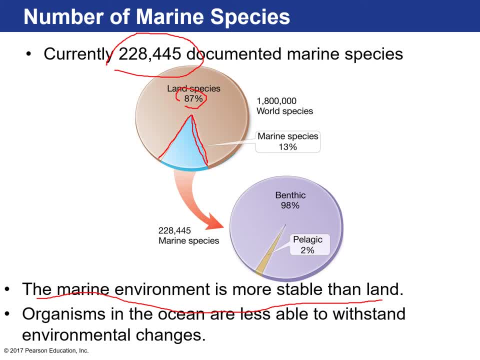 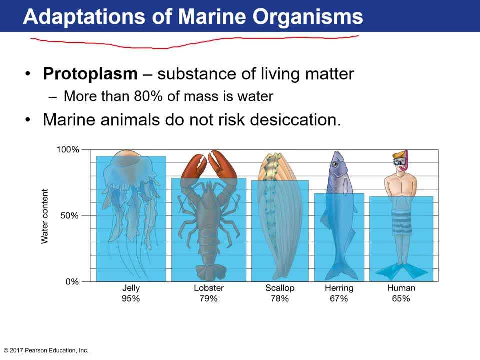 They're not able to withstand major environmental changes. Okay, Protoplasm, all right for the next. I think like 20 slides we're going to talk about the different types of adaptations for marine organisms. Protoplasm is the substance of living matter. okay. 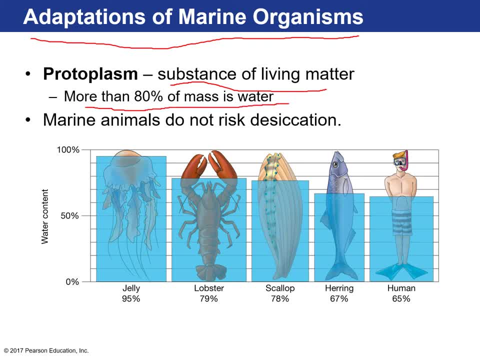 More than 80% of that mass is water And marine animals. in some cases they don't risk desiccation by being in the water. Some marine organisms are made up mostly of water, like jellyfish Humans- about 65% water. 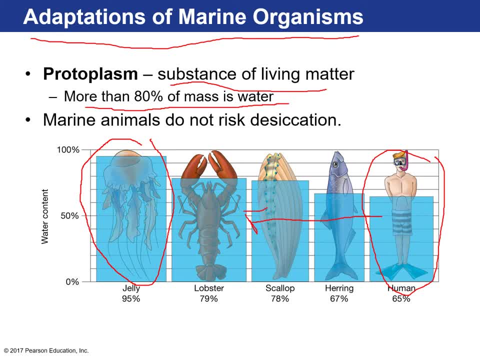 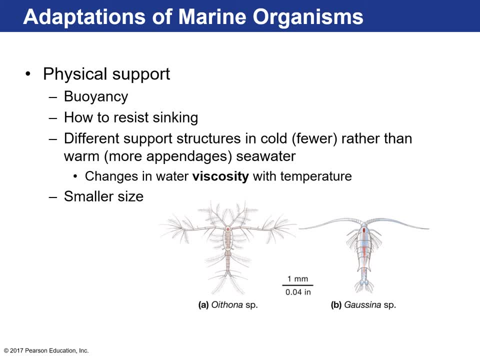 And then it kind of increases in this direction. Okay, So another adaptation for marine organisms is the ability to float in the water. okay, Physical support: Buoyancy is very important. Imagine living in water, right, Like if I was just thrown into the deep end of the pool. you're going to have to start treading water, right? 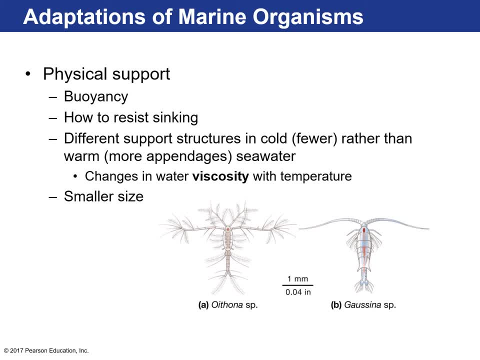 And that can be pretty tiresome. You'd be spending a lot of energy just swimming in itself. So a lot of marine organisms have adapted. They've adapted to different ways to resist sinking and to use the least amount of energy as possible. okay. 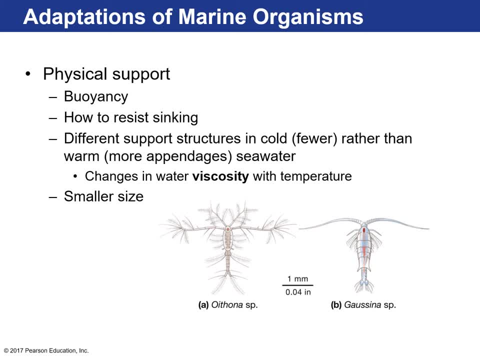 So organisms in different environments have different support structures. okay, So cold water organisms. these are two comparisons of krill in cold water here, and then here is warm water. Well, warm water, the krill have to be a little skinnier and ganglier. 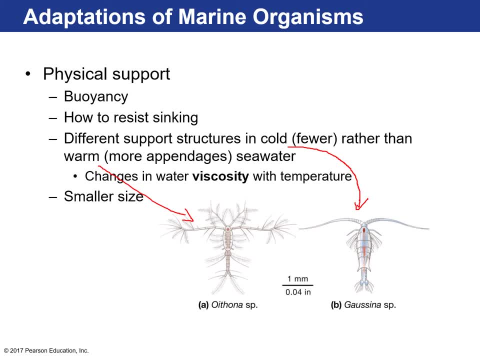 Their appendages stick out a little more to help them float in the water. Okay, So they have to be a little bit thicker to help them float. Why? Because warm water is less dense, And in order to float in less dense water, you yourself have to be less dense and more splayed out, like you see here. 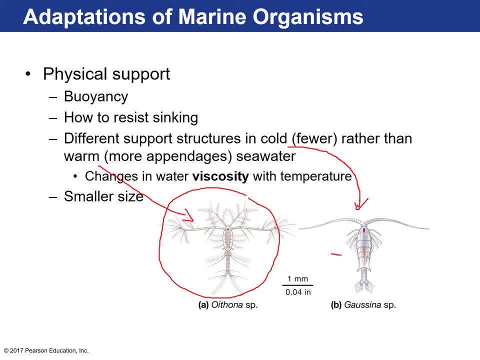 Um, if you're a krill living in cold water like this guy over here, he can afford to be a little thick, little you know, a plump around the edges here. uh, because cold water is denser, So you don't have to be as buoyant in cold water. 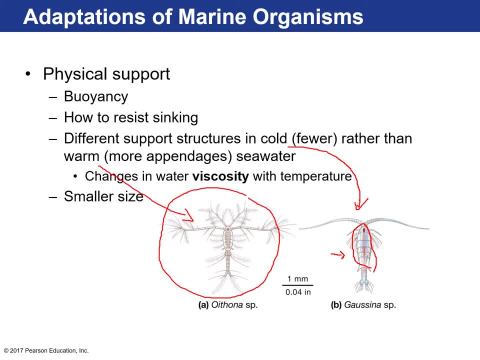 So they're. they don't have as many appendages. They've got a little more meat on them, Okay, So the water viscosity changes with temperature, And so, uh, in warmer waters the krill are smaller, and in colder waters their krill are much larger. 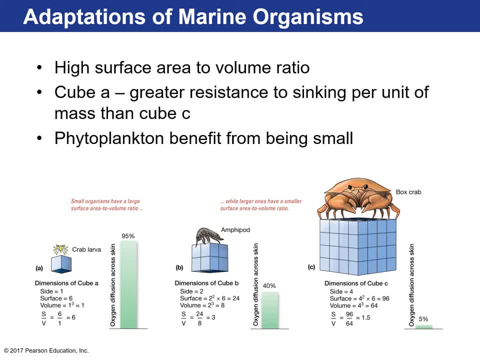 Okay, Another uh uh adaptation for a lot of Marine organisms, uh is is to be really small, especially organisms like algae. Um, if, if your bodies are small, uh, you have a high surface to volume ratio and that's particularly important for the single. 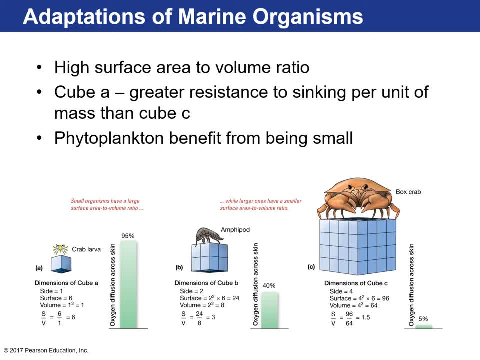 Celled organisms because um a lot of times they uh allow um uh nutrients to kind of diffuse through their bodies, um and then allow waste to kind of move out of it. So if you have a a smaller or a higher surface to volume ratio, that process is easier. 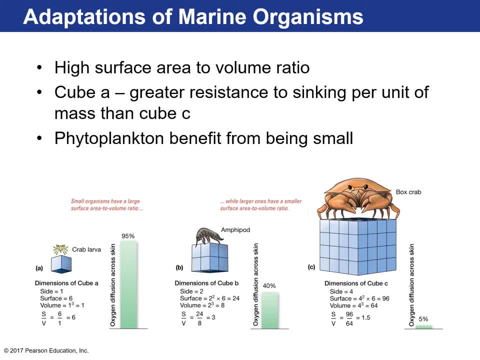 Okay, And then also cube a here. because of that small size, they have the greatest resistance to sinking. So again, then, you use less energy keeping yourself afloat in the sunlit layers of the ocean, Whereas, uh, these guys over here, these chunky guys over here, um, uh, they will sink uh faster. uh, box crab. 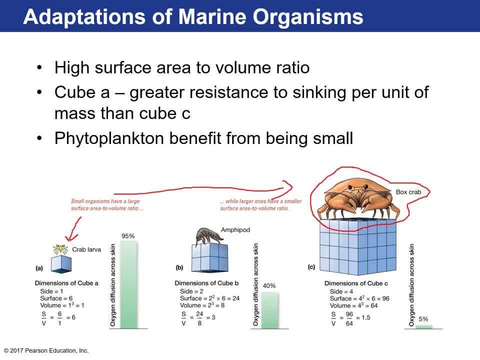 Doesn't care. He's a benthic organism So he's used to being at the bottom of the sea floor. So phytoplankton benefit from being small for two aspects: staying afloat and also being able to pass uh waste and also absorb nutrients from the water itself. 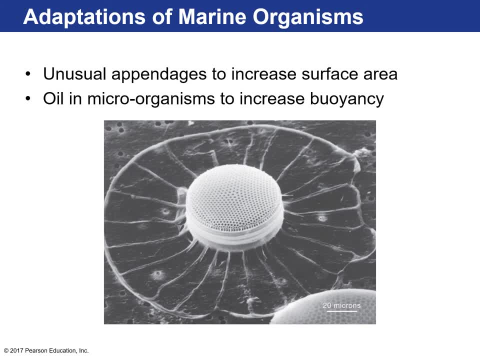 Okay, Sometimes you can, uh, organisms will have kind of unusual appendages that stick out from uh their bodies. This is a, uh, a type of diatom. um, right here, diatoms- uh, we would have used the SEM if not for the global pandemic, but um, here, uh, here's a diatom. 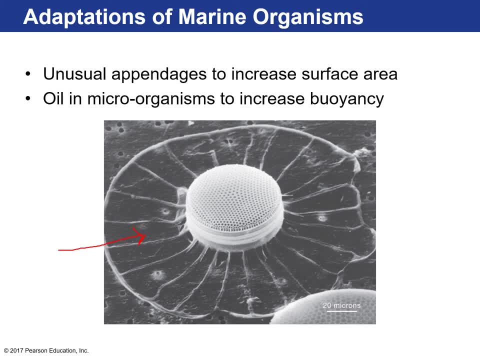 It makes its shell out of silica and this is its test, or it's kind of armor that's surrounded the single-celled algae, Um, and it, you know, photosynthesizes, So the oxygen comes out of those little holes, right? 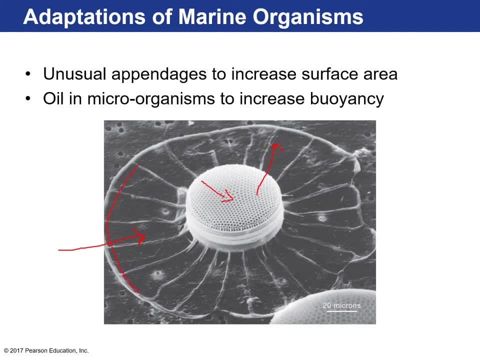 Takes in carbon dioxide, but it creates this appendage to help it float in the summit layer so that it can has the ability to photosynthesize. In addition to that, diatoms also create a little droplet of oil. I don't know if you've ever you ever used that old Italian trick when you boil pasta, where you're like, Hey, just drizzle some olive oil into the boiling water. 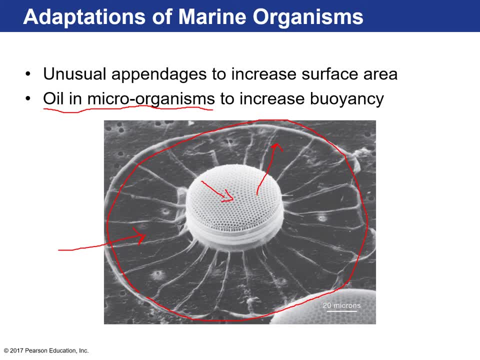 So the pasta doesn't stick to the pan or the pot. Um well, the oil floats right. So, Uh, you can see that oil float. Um, these diatoms create a little droplet of oil within their shells to help them keep them buoyant. 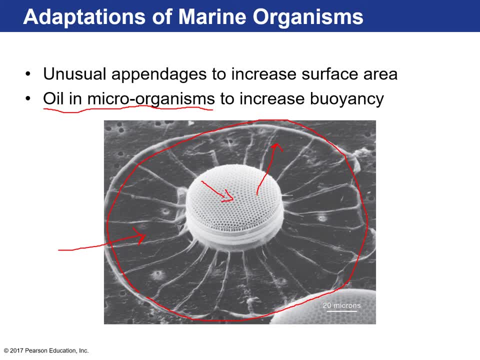 Okay, And a lot of times, this is what? um, when, when these guys live in a certain environment and they die and their shells kind of sink down to the bottom of the sea floor, that oil is what eventually becomes hydrocarbons that we use for energy consumption. 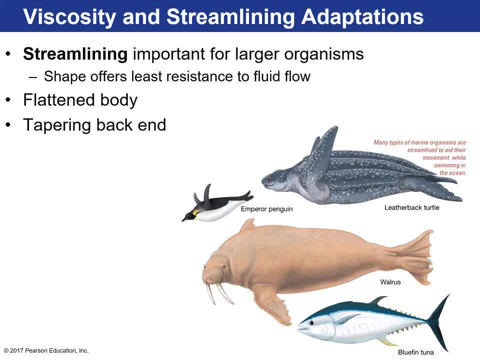 Okay. Another uh adaptation that marine organisms kind of uh uh take is called streamlining. Okay, Streamlining uh is important for larger organisms. essentially, uh make some more aerodynamic. Remember if, when you're living in water, you're living in a viscous fluid. 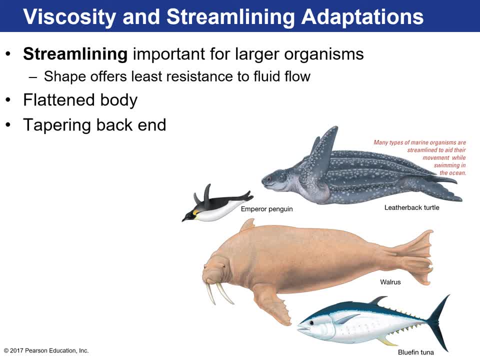 Okay. So you've gotta be able to move through it quickly, quickly, especially if you're trying to catch uh your meal or escape someone uh from eating you. essentially, So, uh, what ends up happening is, Uh, these organisms will evolve. 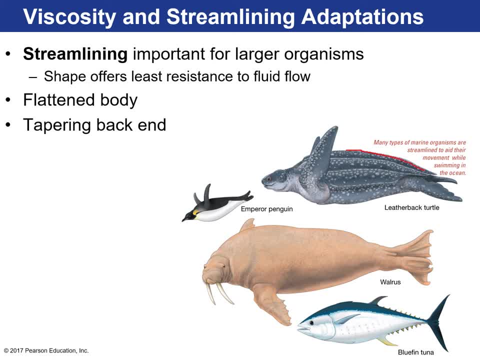 Uh, these organisms will evolve Very similar body shapes, tapering in the back, Okay, Um, flattened bodies, All right, Like you see here, uh, it just offers the least resistance to fluid flow, Okay, So, despite the fact that, uh, this is a reptile here as a turtle, this is a bird, right? 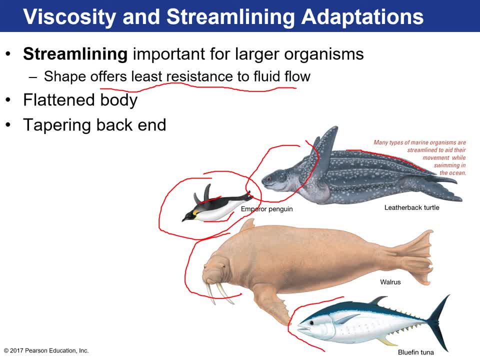 Uh, this is uh a mammal and this is a fish: all organisms that are part of uh uh different branches have all evolved. Uh different branches have all evolved Uh. different branches have all evolved uh into uh streamlined shapes to because of their environment, because of their marine environment. 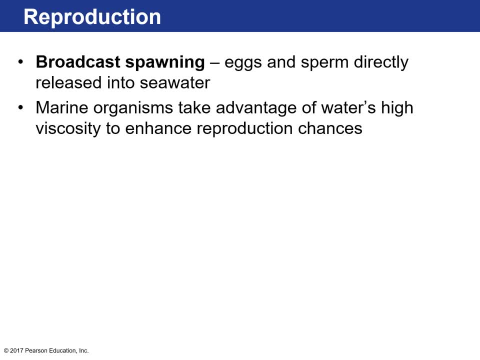 Okay, let's talk about reproduction. So organisms are marine organisms. in the ocean, They often reproduce in this fashion called broadcast spawning, which is essentially just shooting out their sperm and eggs directly into the seawater. Just shit, It's almost like like trees and pollen. 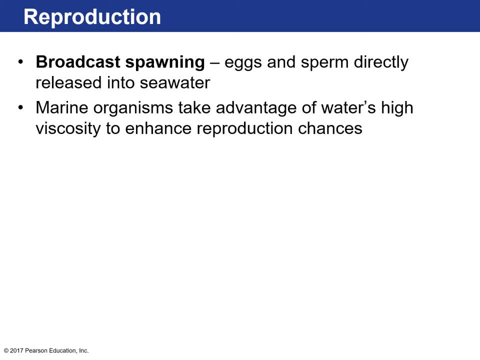 Just kind of Throwing it out there, just letting it go right into the air, into the water. Okay, Um, and so the marine organisms take advantage of that high viscosity of water to uh increase their reproductive chances so that the sperm and uh will run into the eggs and and fertilize them. 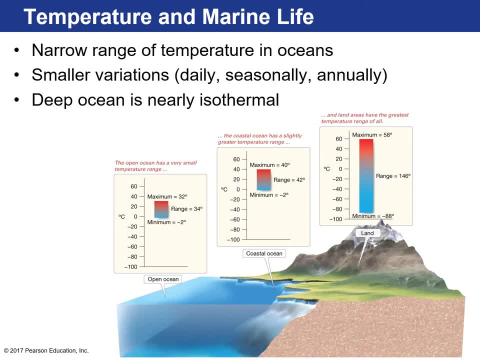 And then and then, uh, as a result of that, Okay, So if we look at, uh, temperature changes in the ocean, um, really, there's, there's a really narrow range of temperatures in the open ocean. Okay, 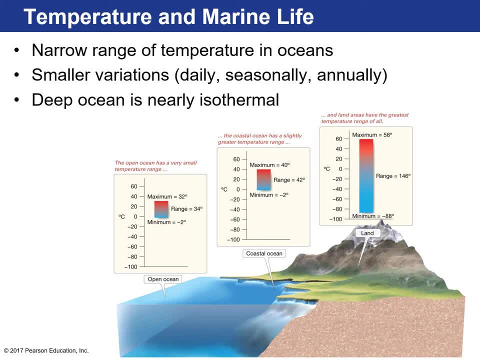 Uh, there are really small variations, uh, in daily temperatures, seasonal, going from uh uh winter to spring, to summer, to fall to winter, um, and then annually, a year to year, the temperatures are very uh narrow. 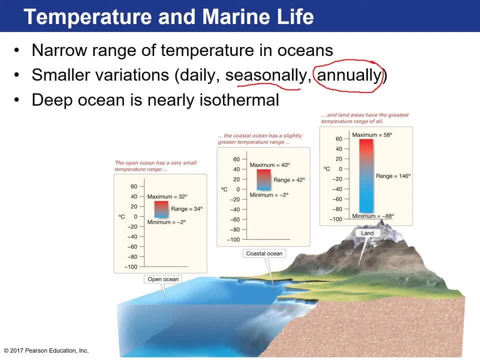 Okay, So here's the open ocean temperature range. Okay, At minimum negative two degrees Celsius, at maximum 32.. Okay, So that range is about 34 degrees And that's open Ocean. Okay, So this is right here: Open ocean. 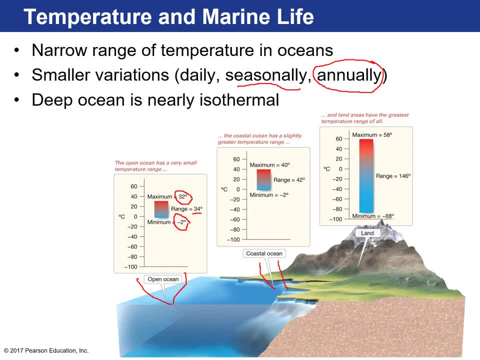 All right. If we go to coastal waters, uh, the range is a little bit higher. It's 42 degrees, So the water gets a little warmer. It doesn't get much colder, So there's a little higher range, Okay. 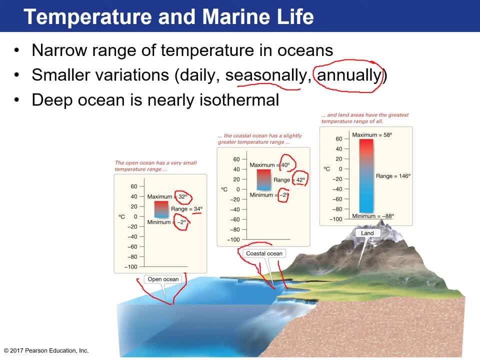 So this environment, coastal oceans, um, differ just slightly. a little more variations, almost like, uh, uh, just about eight degrees, uh, more variation than than the open ocean itself, And that's what leads to more speciation in coastal water. 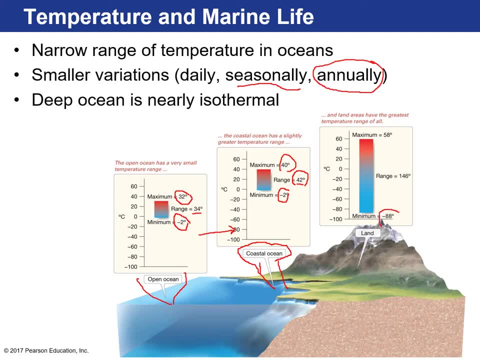 But look at land in the coldest areas. uh, on land you can have negative 88 degrees Celsius. That's really cold, Okay, And at most 58 degrees Celsius. All right, That's like. I think that's about 135, 138 ish. 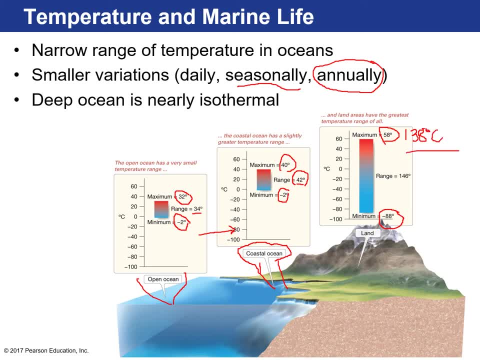 You can test quote me on that later. Um, but that's a range of 146.. Okay, That's three, almost four times the range of, Uh, these environments. So that's why, uh, there are a lot more uh, different, different species that have adapted to the different environments on land and the deep ocean. 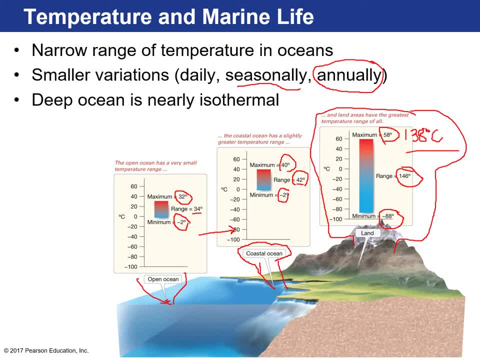 And now this is considering the surface of the ocean, right. If we consider the deep ocean, right Like so, if we go about a kilometer of depth and consider the deep ocean, it's nearly isothermal, meaning that the temperature does not change whatsoever. 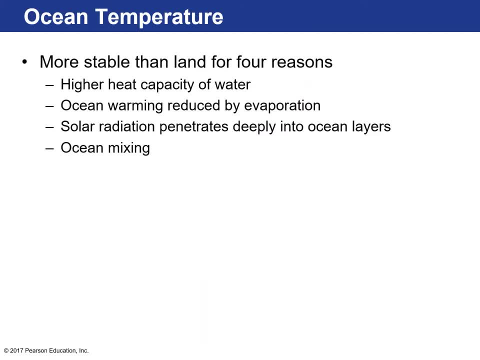 So there's no range, All right. So the ocean temperature is more stable than land for four reasons. One is higher heat capacity. We've talked about that before. water has an ability to hold more heat, Um, and so it takes more energy to change the temperature of water than it does the change temperature of land. 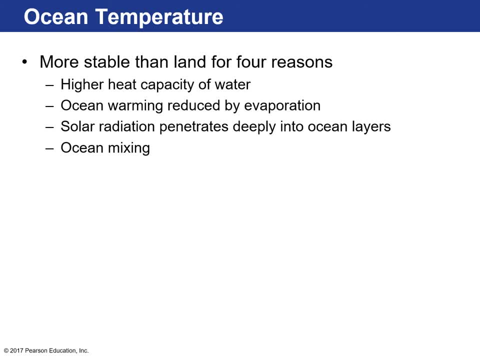 So water kind of uh, the, it's temperature remains stable, even as if you're adding heat to it slowly, land will change much more Rapidly And also, once the heat's in the water, it takes a long time for the heat to be kind of uh or to lower the temperature of water. 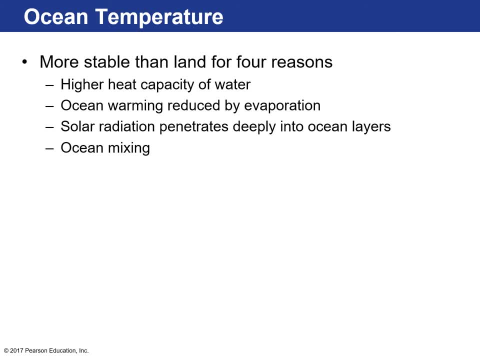 So water kind of resists wild swings in temperature, and that's what high heat capacity is. Okay. Um uh, ocean warming is also reduced by evaporation. So when, on those hot days where there are no clouds and the sun just beating down on the ocean surface, ocean water will evaporate and that removes heat from the water itself. 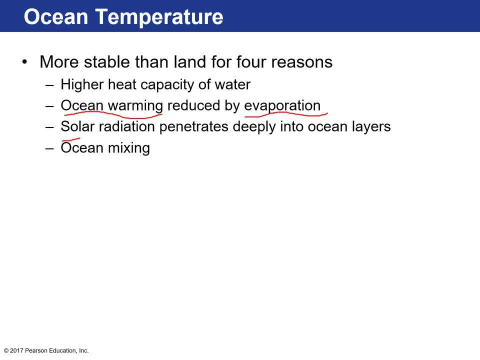 Okay, Um, and the other reason is that, like, solar radiation penetrates not just the surface of the ocean but also the layers beneath it, So the heat is kind of dispersed, kind of uh in depth, Whereas on land, like, say, you have uh like the sun hitting sand. 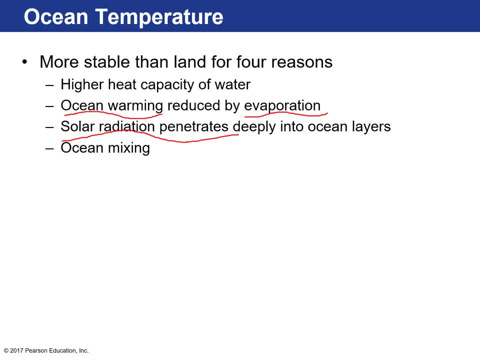 Okay, The upper layer of the sand will be really hot, but you can dig your toes into deeper sand, Uh, and it's much cooler. That's one way of uh avoiding burning your feet Right And, In addition to that, water mixes. 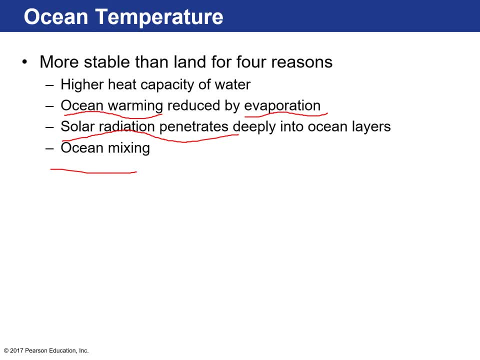 So as a wind pushes the water, some hot water on the surface might mix and start sinking. Uh, and it it's has a three-dimensional kind of mixing factor to it, Whereas land doesn't. it just hits the surface and that's it. 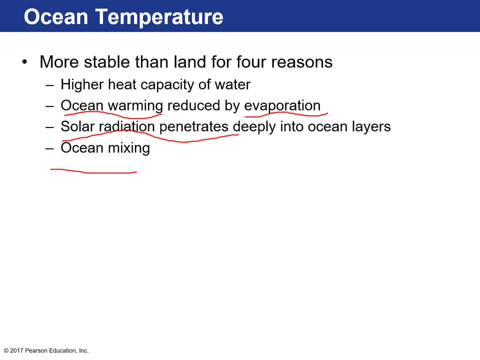 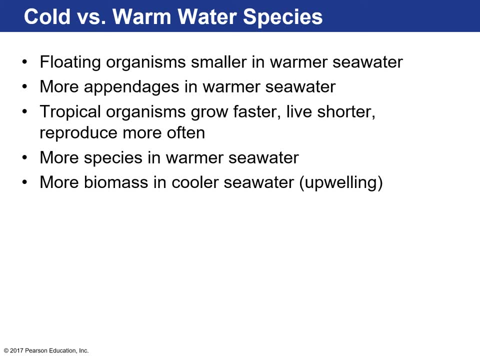 You dig a little bit and it's cold, or it gets much colder than uh in comparison to the surface. All right, So let's compare um cold water versus warm water. uh, Marine species, Okay, Um, Floating organisms are smaller in warmer seawater and that's because of the density of the water is much lower where it's warmer. 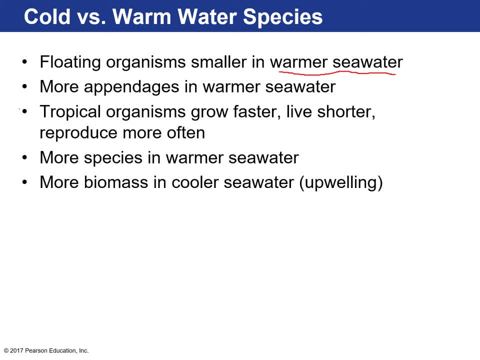 Okay, So they have more appendages. Um and also uh. their lifespans are typically faster- life in the fast lane for those tropical organisms. They grow faster, they live shorter lives, but they were produced more often, Okay. 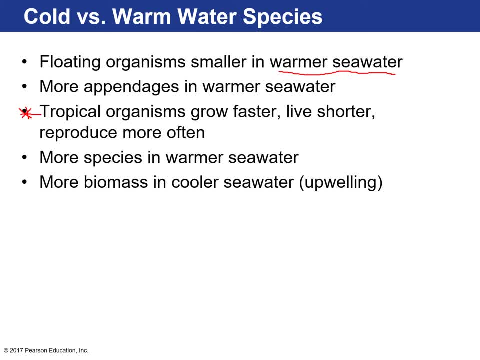 And that has to do with- uh, higher metabolic rates in warmer water. Okay, There's also more species in warmer water. Okay, They have more fluctuations in temperature. Typically, uh, a lot of times warmer seawater might be in shallower areas. 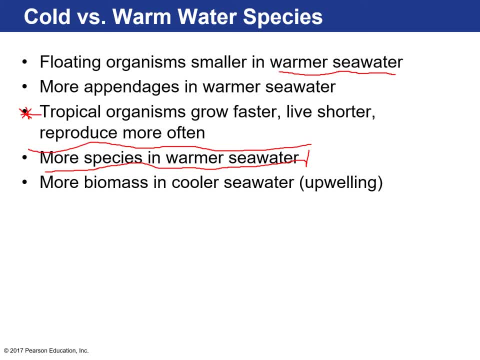 Okay, But in terms of biomass, um, like the massive organisms that exist in cooler seawater, because typically cooler seawater might involve upwelling the kind of uh bringing of nutrients to the surface, uh from the deep, And that sparks a lot of biological productivity. 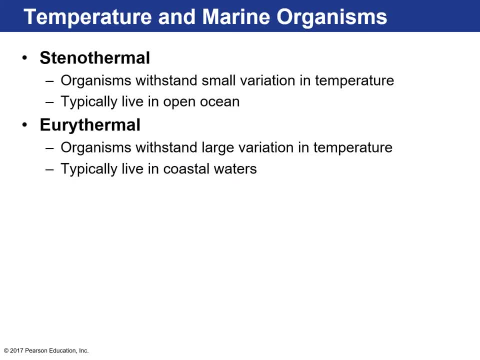 Um and uh, you'll Find A lot more biomass there. Okay, So um organisms can withstand variations in temperature. Some organisms can, um Steno thermal organisms withstand small- ver only can withstand small variations in temperature. 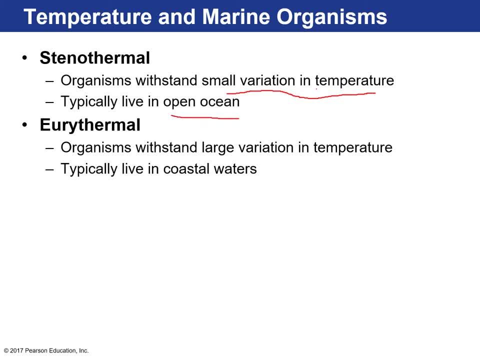 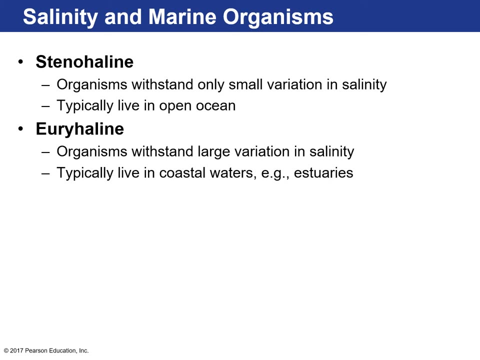 So they're typically open ocean or prologic organisms, Ural, URI, thermal organisms. They can withstand larger temperatures. Um, and they're typically coastal water organisms, So they can withstand large variations in salinity. All right, And then the same kind of definitions fall for uh uh, salt. 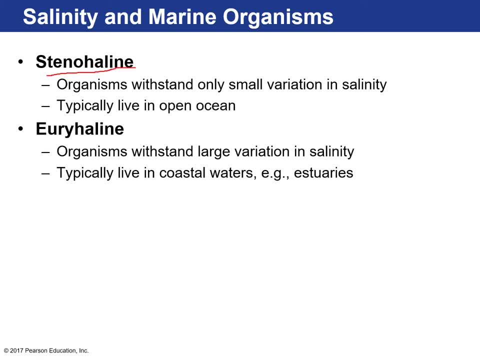 Okay, So Steno Haline organisms are ones that can uh um, only withstand small variations in salinity. Again, those are typically open ocean organisms, and Euro Halene organisms can withstand large variations in salinity. So your estuaries, wherever you have uh river water in fluxing into the ocean, that will. 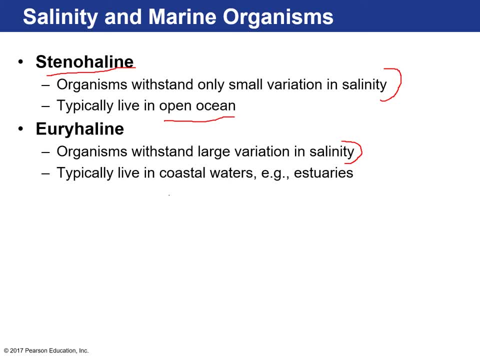 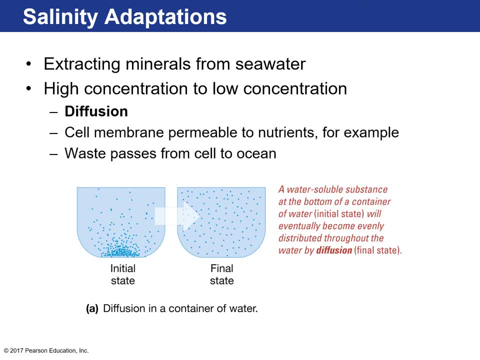 chains the salinity there. coastal waters, those organisms that live in these environments, are urohaline. Okay, so some organisms extract dissolved solids directly from seawater. Some examples are diatoms with silica or SiO2 and coccoliths with calcium carbonate. 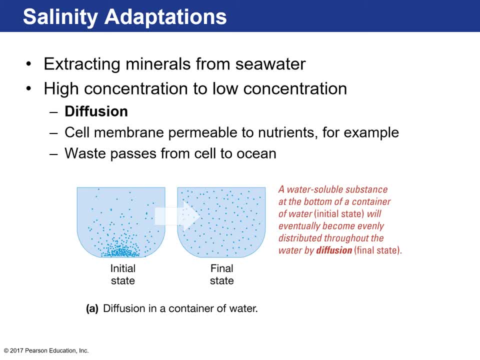 They'll remove calcium directly from seawater. Okay, so that's how they extract components from seawater And some components of seawater. they can diffuse through the water, especially like nutrients or waste products, And diffusion essentially, is how these either nutrients or waste. 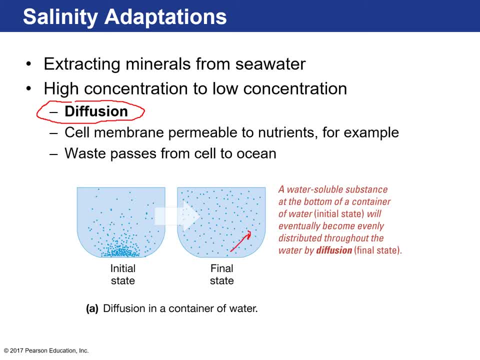 are removed from seawater And so if you have a seawater you can kind of move through the water And so they disperse and space themselves out evenly. So they initially start off really concentrated, but over time diffusion. 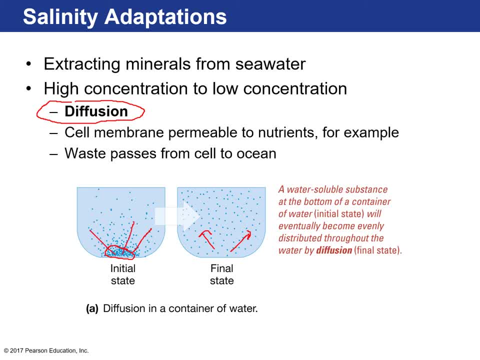 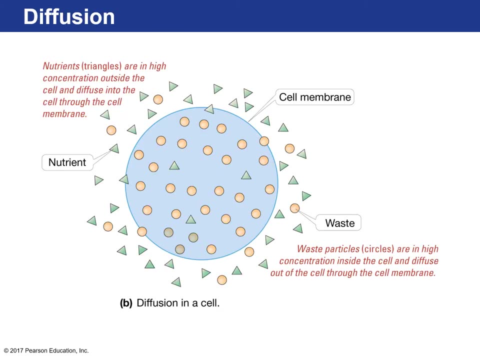 in a container of water will space out and even it. Okay, so cell membranes are permeable to nutrients. Okay, that's a type of diffusion And waste passes from the cell into the ocean via this process. Okay, so here's diffusion, There's a cell membrane, Nutrients. 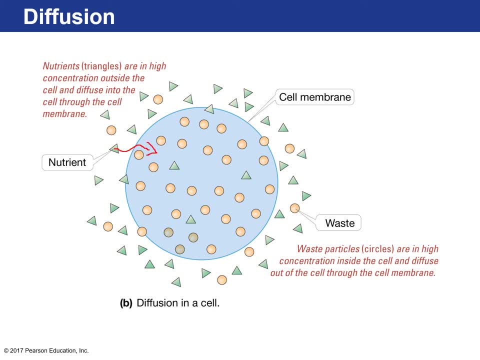 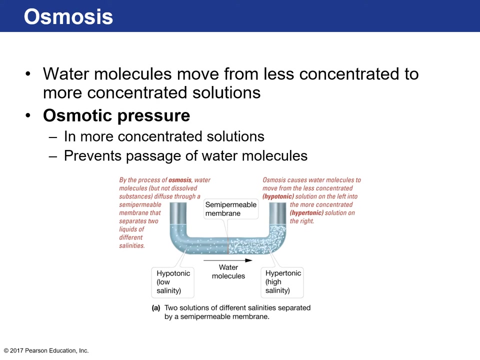 are able to come in. These are usually typically a single-celled algae- Okay, and the nutrients come in and then the wastes are allowed to come out And essentially they just diffuse through the cell walls or cell membranes. All right. osmosis, essentially, is how water molecules move from membranes or 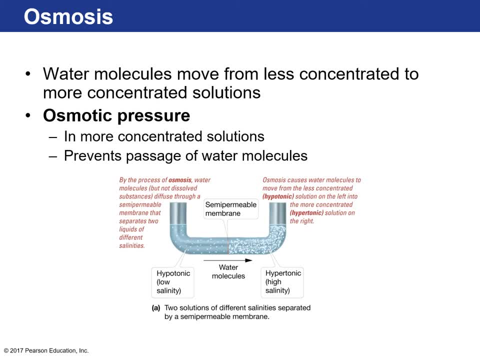 water that have less concentrated or more concentrated solution. This creates osmotic pressure. So say, you have two liquids, Okay, and here we have a semi-permeable membrane, which may be a marine organism, for example, And then we 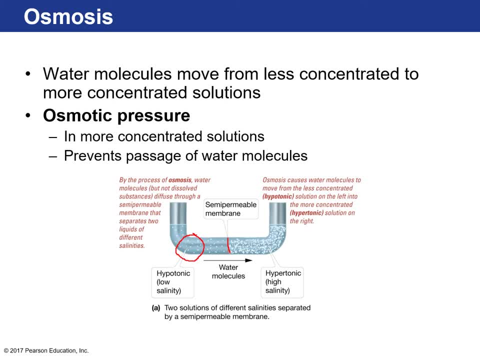 have a solution here that has low salinity. We refer to that as hypotonic, Okay. and then we have a solution over here with really high salinity- We'd call that hypertonic, Okay. and so what happens is because of the diffusion water. 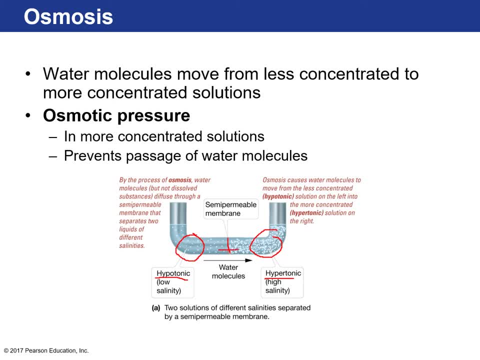 molecules will move through the membrane into the high salinity solution in order to even out the two liquids. Okay, so salinity itself, like the actual dissolved solids, can't travel through the membrane, but water will, And so the water will move towards the hypertonic solution to even out the salinity levels in both. 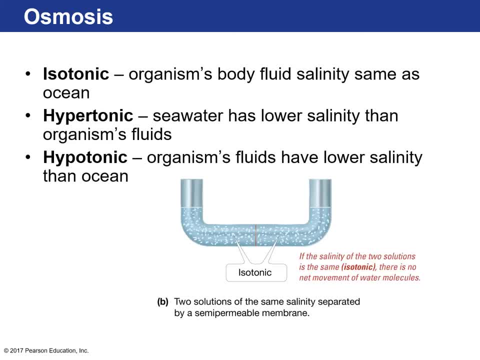 these solutions. Okay, so when you have an organism or a marine organism, isotonic means the organism's fluid salinity is the same as the ocean, And that's a good concept for the organism. Okay, so that it's not losing any water from its cell membranes. 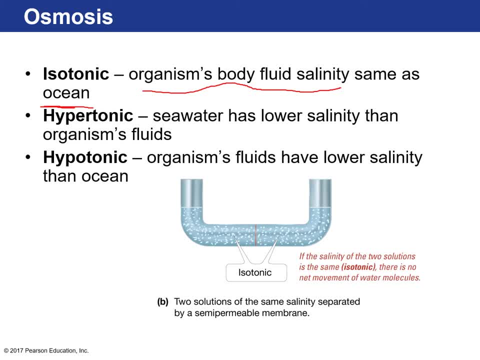 and that it's not taking in any water. However, essentially this is an isotonic, an example of isotonic: where the liquids in this area are, it's the amount of water that was ill-conditioned. liquids in this area have the same salinity as the liquids over here. okay, 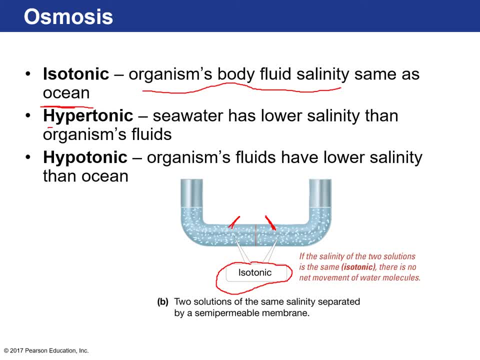 so that's good, all right, that's good for the organism. but if you have something that's hypertonic- that means seawater has lower salinity than the organism's fluids- okay, and if that's the case, the organism is going to start losing water molecules to the surrounding water and it's going to kind of prune up. okay if? 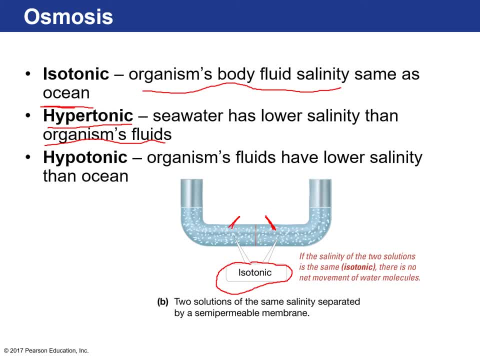 the organisms fluids. organisms fluids have lower salinity than the ocean. okay then that means the water molecules are going to move into the body of the organism and the organism can actually kind of explode. okay, so if you say you have a freshwater aquarium and you put a saltwater- kind of hermit crab or 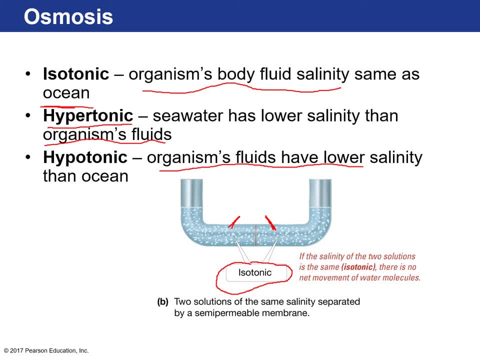 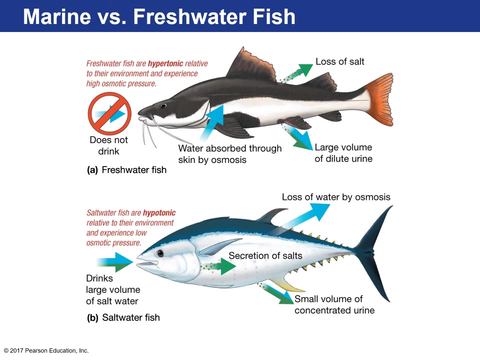 something into that aquarium, it's going to explode because the salinity of the organism itself is higher than the surrounding water it's in, so water molecules are going to move inside of its body and then cause the organism to kind of explode as it seeks equilibrium or as it or an isotonic solution. okay, yeah. 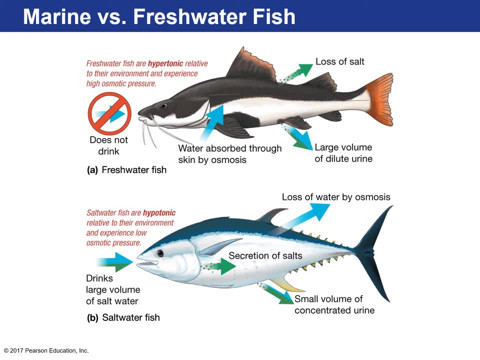 they're very high maintenance. if you're going with saltwater aquariums, all right. let's discuss marine versus freshwater fish. freshwater fish do not drink the water they're swimming in the waters of, absorbed through their skin via osmosis. via this process and the way 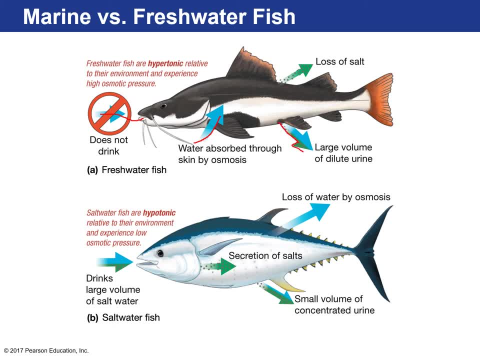 they equalize it is by releasing a large volume of really dilute urine. okay, and then if we look at organisms or saltwater fish, typically in the in the open ocean, this looks like a yellow fin tuna. they drink large volumes of seawater as they swim and then they in. 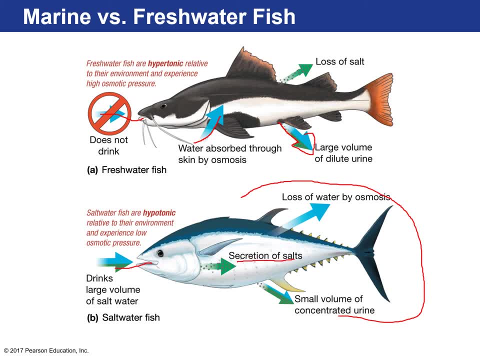 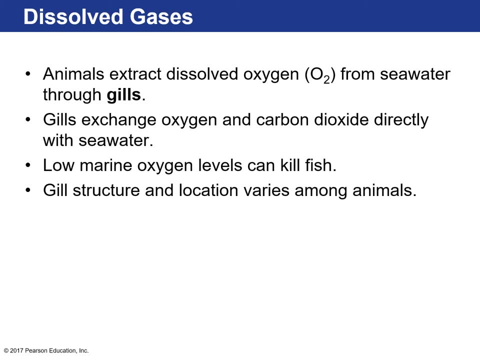 secrete a lot of salts and they release really small volumes of concentrate. Okay, so how do the dissolved gases or how do these organisms kind of respirate or absorb these dissolved gases that are found in the water itself? So marine animals extract the dissolved oxygen through seawater through their gills, and the gills exchange oxygen and 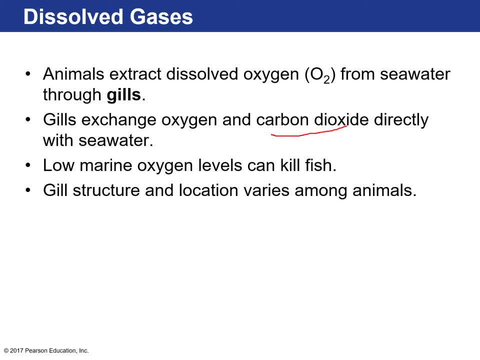 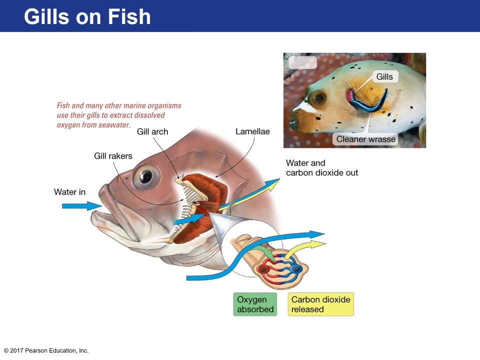 carbon dioxide directly with the seawater. Okay, if you have low marine oxygen levels or dissolved oxygen levels, that suffocates the fish and they die. and the? the gill structure itself and its location varies among different organisms, but here's a kind of a typical. 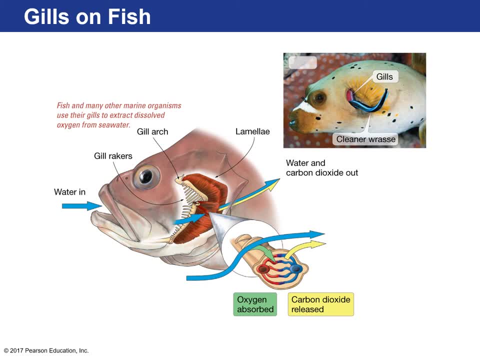 reef fish here. Here are the gills, the gill arc, here are the rakers. so it opens up its gills. seawater goes in through the mouth and out through the gills, all right, and then so this seawater that's filled with dissolved oxygen comes in. 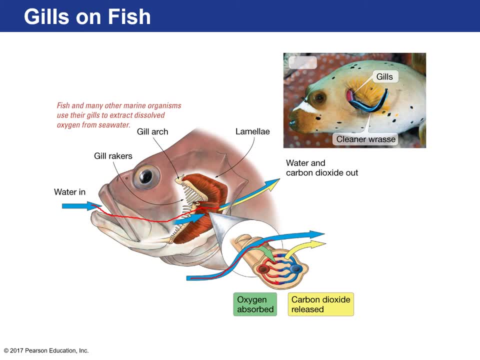 and then the. the oxygen is absorbed by the blood vessels within the gills themselves right here. So water and carbon dioxide comes out of the gills and then the. the blood here absorbs the oxygen- dissolved oxygen- from the water and then releases carbon dioxide. Okay, another 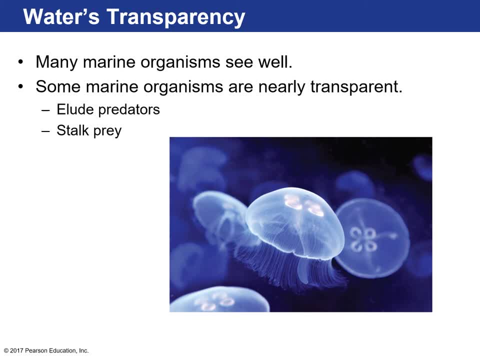 feature, a cool feature. adaptation of marine organisms is transparency. Many organisms see very well in the ocean so if you're kind of camouflaged or see-through, that's very difficult to see. So some marine organisms are nearly transparent, like you see here in these jellyfish. 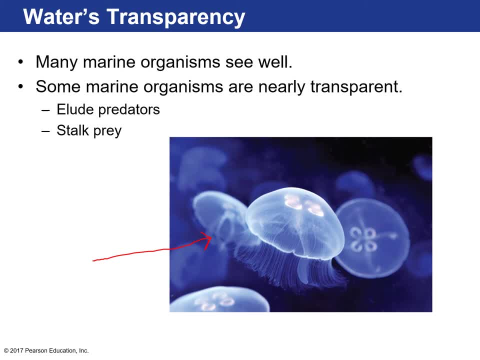 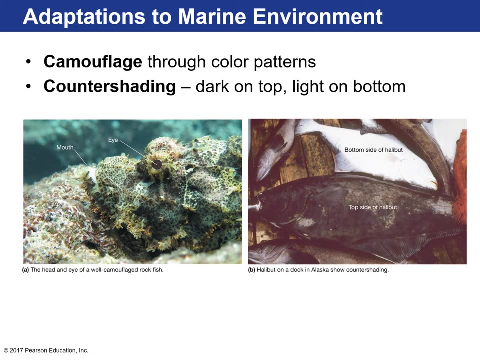 They. they want to avoid predation and avoid being seen. so being see-through kind of helps. It helps you elude predators and in some cases, uh, stalk prey All right. camouflage is another neat adaptation in the marine environment. You can see this here in a rockfish. They're well camouflaged. 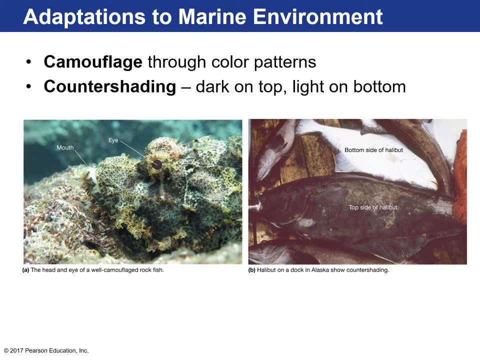 to look like a coral reef or rock that you would see surrounding a coral reef environment, The various color patterns, and then a fish might come near it and then it just lunges at you And then counter shading. Counter shading is very helpful where you have. 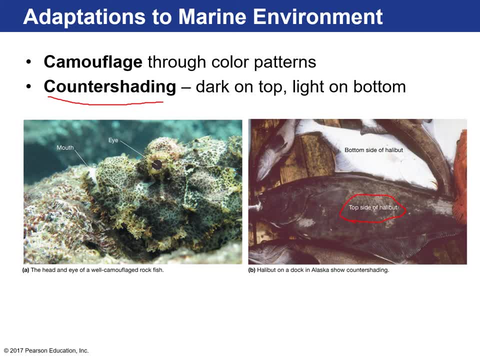 this is a halibut. uh, the top side of the halibut is dark and then the bottom site is the side- is light. You see this in other organisms. Sharks are the same way: dark on top, light on the bottom. So if the shark passes above you as you're looking up in the water column, if you would look up that way, 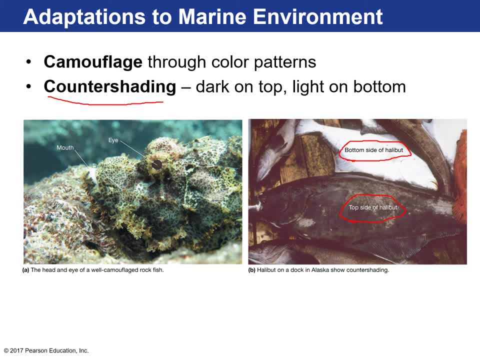 it would look more white because you'd be seeing the sky and the upper layers of the ocean, So the white bottom part of the shark, kind of camouflages, if you were looking up, And if you're at the surface of the water looking down, it's very dark. 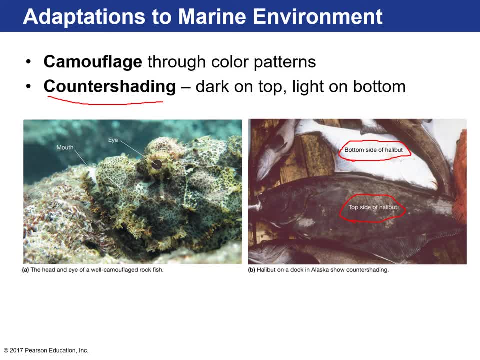 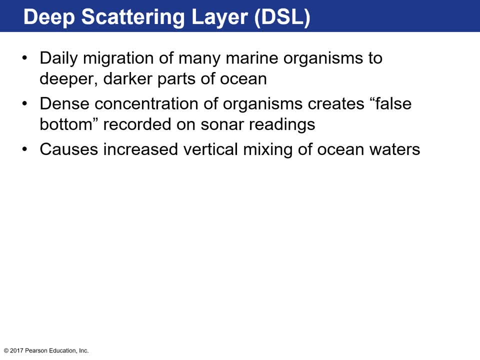 So the top side of a shark is dark and so you would have trouble seeing it as well. So the counter shading is very useful for a lot of marine organisms. Then some organisms do this daily migration called the deep scattering layer or DSL, Okay, and so many marine organisms during the daytime migrate down to the dark. 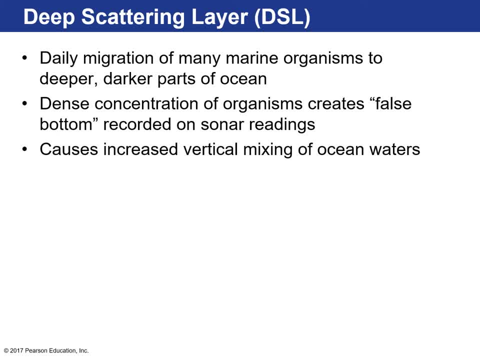 parts of the ocean. Okay, and the reason why we call it the deep scattering layer is because when we do like, when we, when boats use sonar, a lot of times they send out a signal and they hit a false bottom or a sonar reading because of the dense. 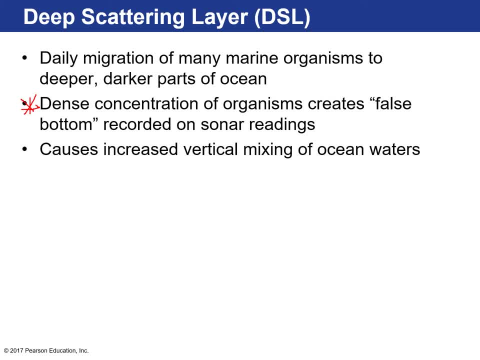 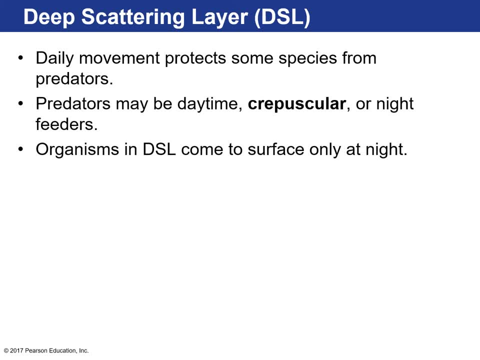 concentration of these marine organisms that are essentially hiding during the daytime. Okay, this causes increased vertical mixing of ocean waters by this daily migration. Okay, and essentially so, what happens is these organisms, during the daytime, they sink down to where the light doesn't penetrate anymore so they can elude predation. and then, when the sun goes, 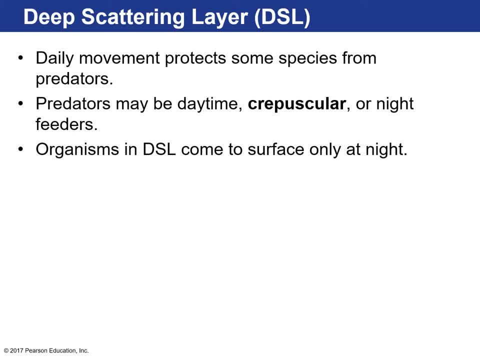 down and it becomes nighttime. then they rise towards the surface and feed. Okay, and they feed on all the auto producers and algae and plankton that are on the surface of the ocean. Okay, so those daily movements protect those species. You may have daytime predators or nighttime feeders. 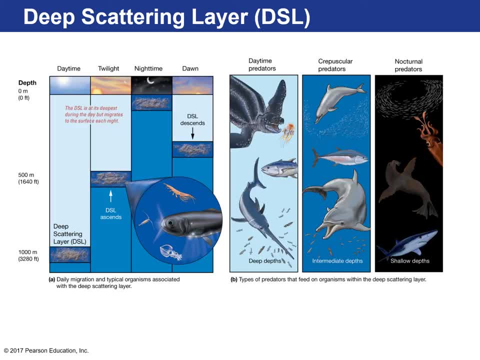 We refer to them as crepuscular. Okay, so here you go. here's the daytime. this is the deep scattering layer, typically about one kilometer of depth, and then, at twilight, it starts to ascend upwards, and at night time, these organisms are up here feeding. right. it can be, uh, some krill, different types of krill, um and oh. here's the. 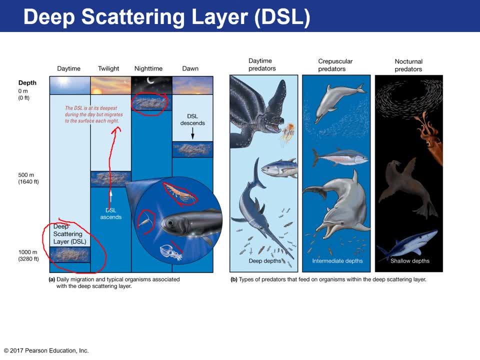 grill, sorry, um, and you know uh squid, larvae and fish. Okay, um, if you have uh night nocturnal predators, squid or nocturnal predators- you're going to have a lot of fish that are going to be active in your environment. There's also the night time predators, like sea turtles, and then 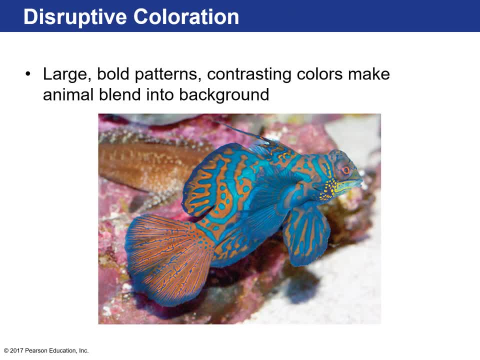 crepuscular predators like dolphin or bluefin tuna. You can have just daytime predators like sea turtles. All right, there's also disruptive coloration. that's a um, a really nice type of adaptation. uh, beautiful. A lot of times they might have circles back here to make you think that. 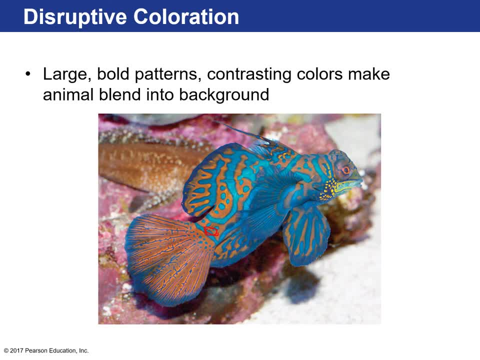 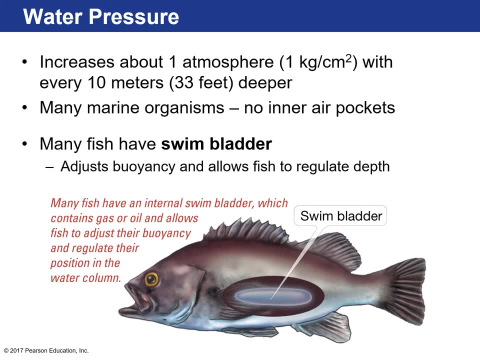 they're eyes in the back of the body. Okay, so, uh, these bold patterns and contrasting colors help to make you think that they're eyes in the back of the body. Also, there are many specific adaptations towards water pressure. So when organisms, marine organisms, want to like uh kind of rise up to 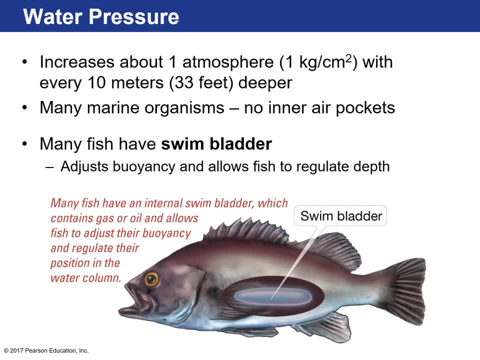 uh, lower pressures or upper layers of the ocean or sink down to deeper layers. um, they've evolved to have this uh organ called the swim bladder. Okay, the pressure if you go um, uh, the pressure increases about one atmosphere every 10 meters of depth. Okay, 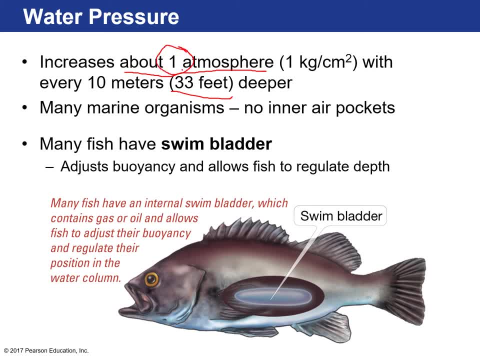 So this is the pressure we feel at sea level. So if you were to go down 33 feet deeper into the water column, you'd feel two atmospheres of pressure. Okay, so, um, many fish have a swim bladder and that helps you adjust buoyancy and allows fish to kind of regulate where they want. 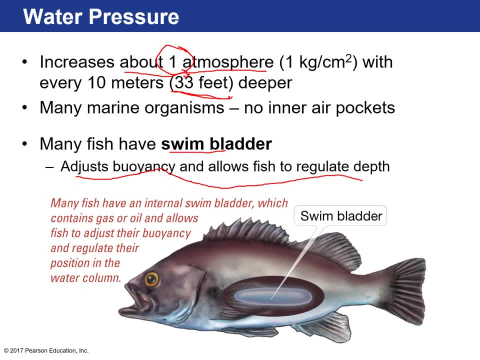 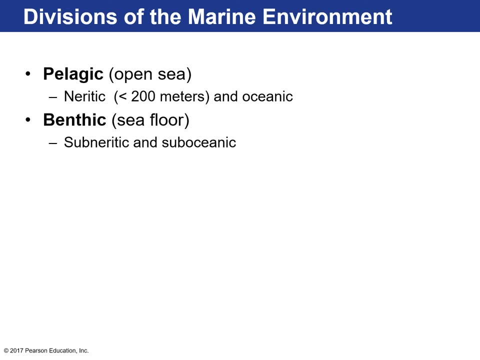 to be in the water column. It's kind of like if you're scuba diver, it's the vest that you wear, the BCD that you fill and with air to adjust your buoyancy. It kind of works in the same manner. Um, okay, let's start discussing the divisions of the marine environment. Okay, the pelagic means. 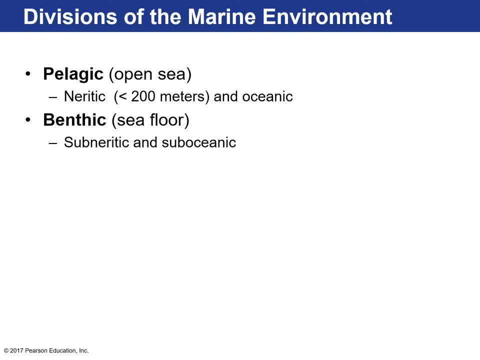 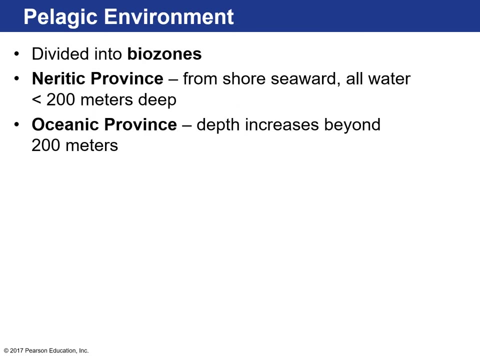 the open ocean- I think we've talked about this before- um, and that's anything beyond 200 meters of depth. And then neuritic means closer to the continents- uh, less than 200 meters, Okay. and then anything benthic means the sea floor, Okay. and then the pelagic environment is divided up into: 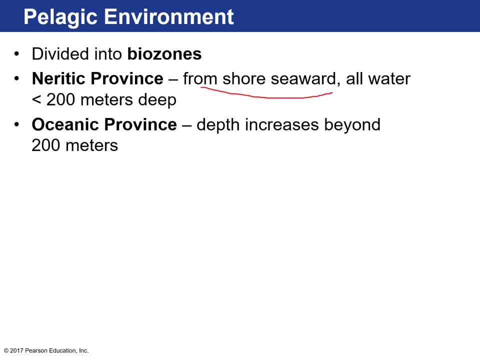 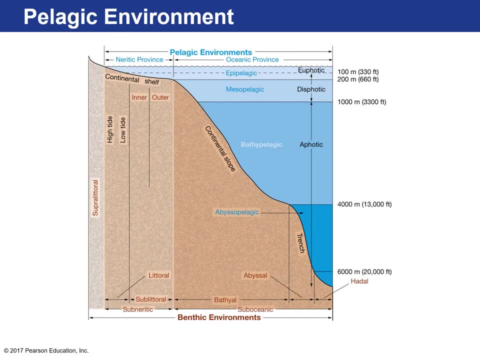 different biozones. The neuritic province, that's closer to land, Okay, and the oceanic province is way out into the, uh, open ocean, Okay. so here you can see the different environments. Okay, here's the neuritic province, very close to land, Okay. shallower waters: sunlight typically reaches all. 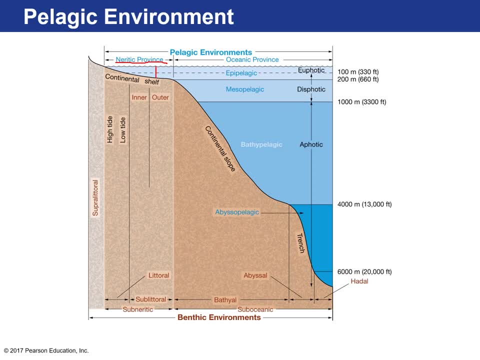 the way down to the sea floor, Okay, um, here's your ocean province, All right. all the way out here, beyond kind of greater than 200 meters and deeper, Okay, um, and then here, this is your, what we refer to as the euphotic zone. This is the upper 100 meters, or 330 feet of the entire ocean, And this 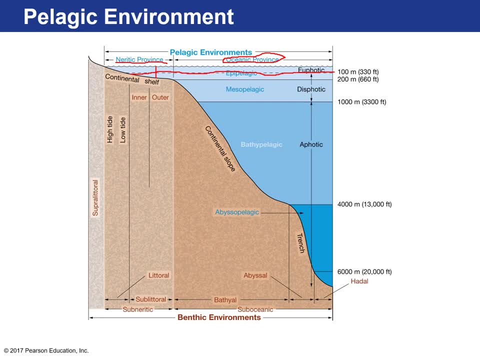 is where the majority of photosynthetic organisms live: above this layer, because that's where it gets enough sunlight to photosynthesize, And then below that, at about 660 feet. that's the epipelagic zone, Okay, and that's where, uh, essentially most of the photosynthesis occurs. So it has a maximum of in this area, but the entire 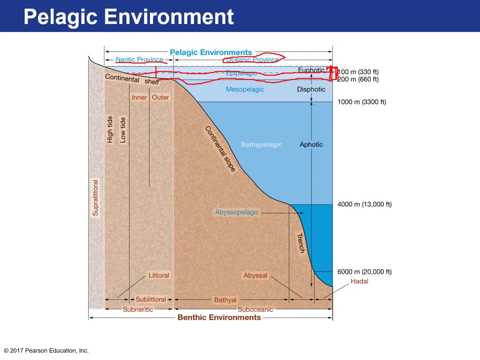 area goes up to about 200 meters. That's essentially um as far as photosynthesis occurs, The mesopelagic zone, um. this dispersed light can make it down here. It's very dark here, but you can get uh light that, like very diffuse light, make it into this area. 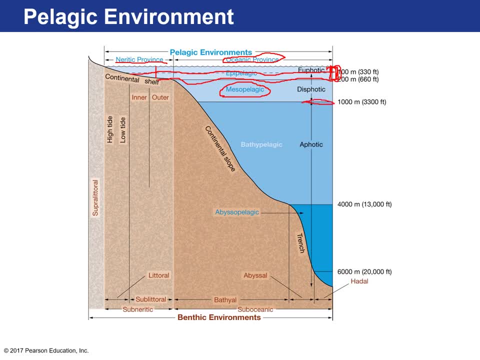 And then, once you get beyond, uh, this layer, it's complete darkness. That's the aphotic zone, Okay, and we refer to this as the bathypelagic area. And then, once you get even deeper areas, this is the abyssopelagic area. 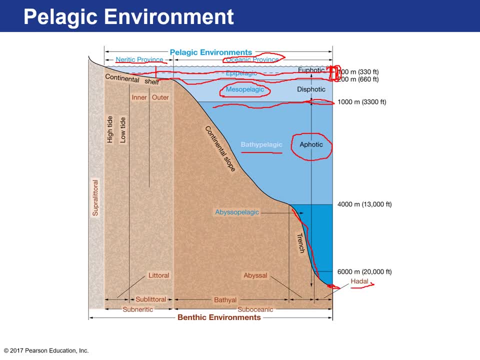 And then down here at the lowest parts of the ocean, we call that the hadal zone. Okay, so here are the different distinctions for the benthic environment. So that's on the sea floor. This is the abyssal. Okay, um, here are the uh inner and outer, uh subliteral zones. 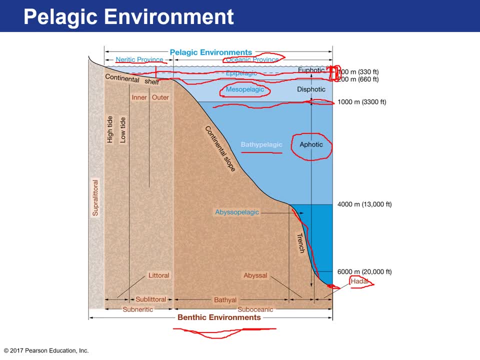 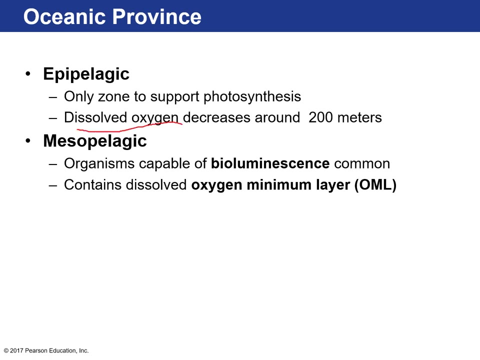 And then here are the um, uh, superliteral zones. that's above the ocean, But high tide can come in and uh inundate those areas and all that Okay. so the epipelagic zone is the only zone to support photosynthesis. Dissolved oxygen actually decreases around 200 meters. Then it's the 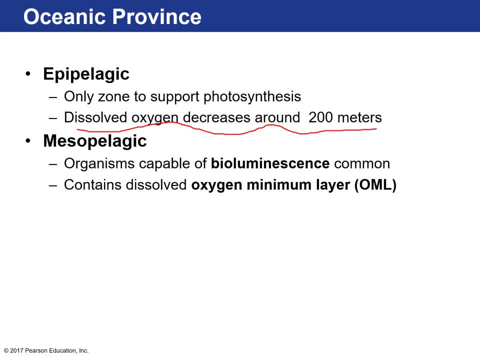 mesopelagic zone. Here organisms are capable of bioluminescence, which is very common. They create their own light. They do that for their own reasons: to catch prey, to attract a mate, because they're so lonely in the darkness Right um and the mesopelagic zone also. 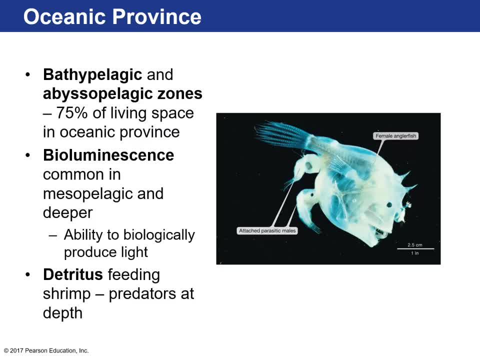 contains, uh, an oxygen minimum layer. Let me show you. I think I have a graph in a little bit. And then when you get to the bathypelagic and abyssopelagic zones, this is the really lower parts of the ocean, So bioluminescence is very common. This is the 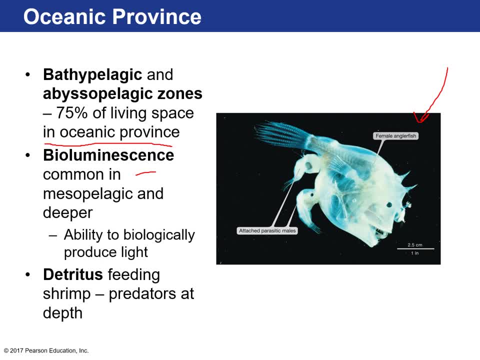 the angler fish. They're capable of bioluminescence- Excuse me, Um, so that's that ability to to produce light, And organisms that live here typically feed on detritus, which is um material, that just organic material that rains down on them from the upper. 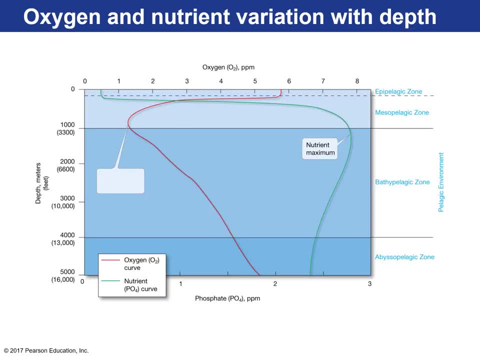 layers of the ocean. Okay so, here's the oxygen and nutrient variation with depth graph. Okay so, and here are the different zones. Here's the epipelagic zone: mesopelagic, bathypelagic and abyssopelagic, So really deep Um, this is phosphate, or, uh, an. 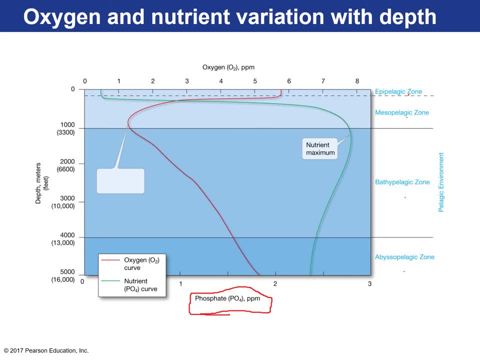 abyssopelagic zone. It's a nice way to measure nutrients, okay, in the water, which are important for many organisms, especially in the upper layers of the ocean. And then, uh, the red is the oxygen curve. So the the dissolved oxygen in seawater is really high in the epipelagic zone. Why? Because 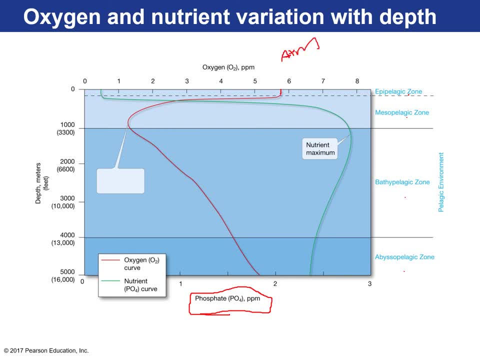 the atmosphere is right here, ATM right, Um, and so, uh, there's a lot of mixing here, A lot of oxygen that's uh put into the upper layers of the ocean because of the atmosphere Steadily declines, okay, and it reaches kind of an oxygen minimum zone right around here. 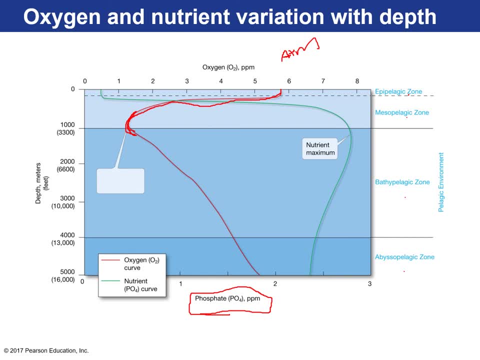 And the reason is because, uh, all those organisms that photosynthesize, when they die, their bodies start decomposing down in these layers and the bacteria essentially use up all the free oxygen as they're decaying away those those organisms. Then the oxygen layers slowly increase as you move into. 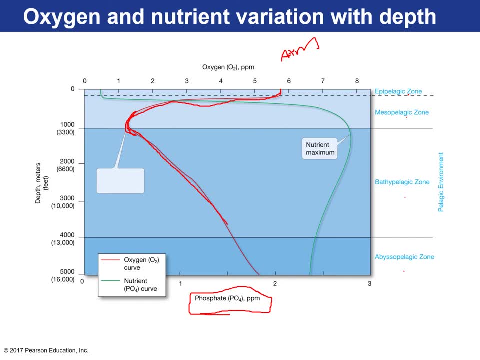 the epipelagic zone. okay, The nutrient layers are very low at the surface and the reason why the nutrient layers are very low at the surface is because you have a lot of those uh, algae and autotrophic organisms on the surface of the ocean And they're using up those nutrients because 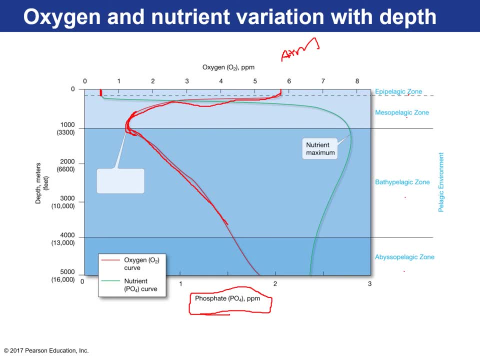 they're photosynthesizing, they're using nutrients, they're creating oxygen, they're living, they're getting eaten by zooplankton and all that. And then, as the populations of those organisms diminish, nutrient levels slowly rise into the surface of the ocean. And then, as the populations of those organisms diminish, nutrient levels slowly rise. 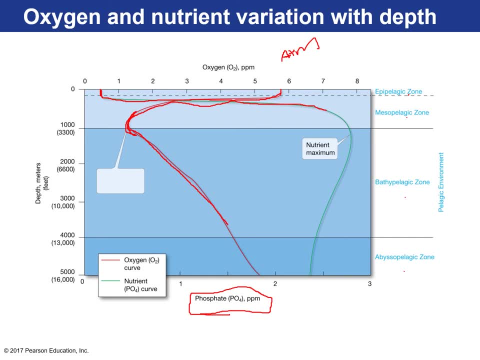 to these layers where there's no, where there's no photosynthesis, and then you hit like a nutrient maximum over here And the reason why the nutrients increase in this direction is because that bacteria is breaking down those- uh those- dead organisms and returning the nutrients back into the water. 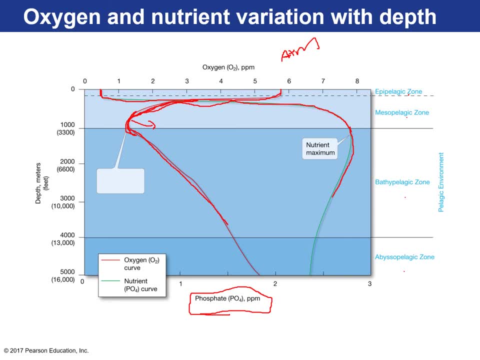 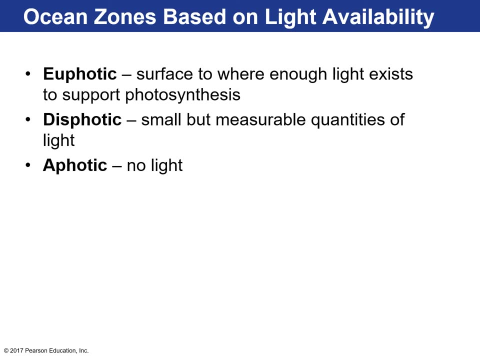 Okay, so you hit a nutrient maximum here and then it kind of evens out as you go into deeper waters. Okay, so then there's- uh, these are the zones based on light availability. The euphotic zone is where light exists to support photosynthesis. Dysphotic zone we talked about 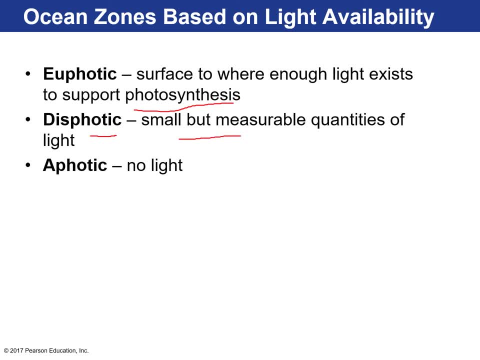 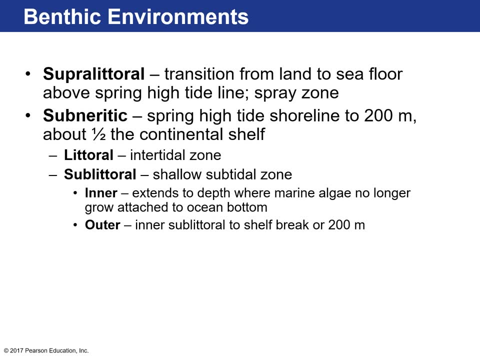 before, That's where they're small but measurable quantities of light. And then the aphotic zone is where you have no light And I showed that in the last image. Okay, and then with the benthic environments, just to kind of wrap this talk up, the super literal zone is the transition from